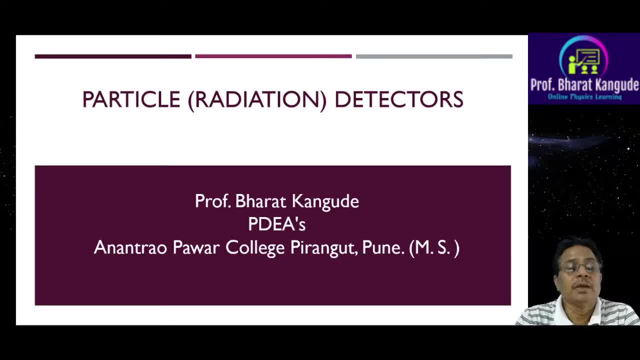 Dear TYBSC friends, in the chapter number four, that is, particle accelerators and detectors. This is the last part of this chapter number four and this title is particle radiation, or particle or radiation detectors. Now, in earlier case, as we have seen, there are several. 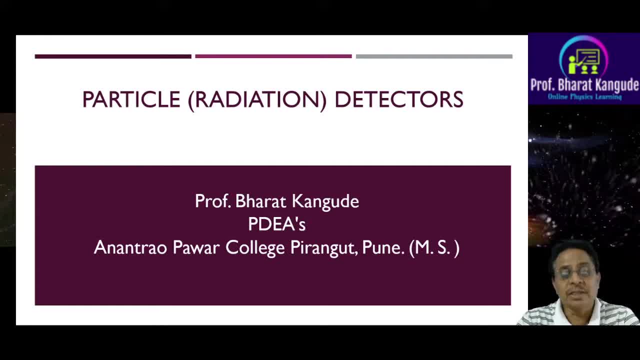 devices which are used to increase the energy of the particles coming out of the nuclei may be alpha radiation, alpha particles, beta, gamma- not gamma, but charged particles, alpha, beta- then some other types of charged particles like proton, etc. these particles can be accelerated and further. these particles can be used to carry out the further types. 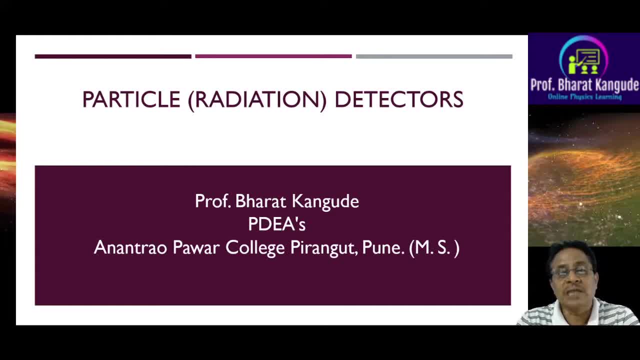 of nuclear reactions, and once such type of nuclear reactions are created or generated, in that process large number of other types of particles are generated or created. Now it is not that easy to identify all these particles. what are the particles that are as an outcome came out of that reaction? and for detecting these particles or this type of outcome of any nuclear 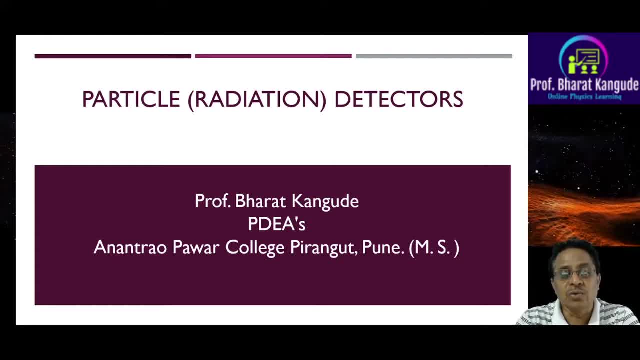 reaction. we require this detector. So very easily one can understand why detectors are needed. so there are some specialties of these detectors. we are going to see their types. we are going to see their functions. we are going to see two such specific examples of such type of detectors. 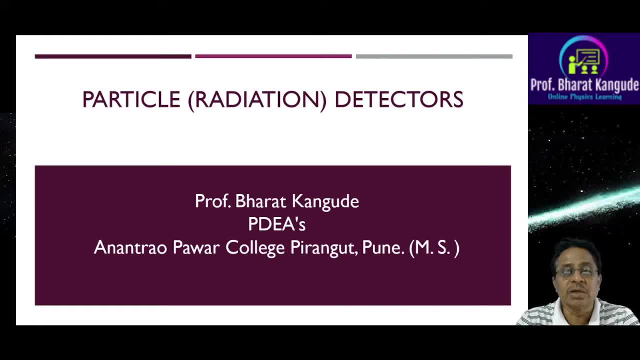 In case of example, this particular device has nine or more types of particles that are present in the nuclei, so that is one means that we are going to be able to understand the particles in each of these types of particles, And so that lets us see the particles that we are coming in contact with, and that helps. 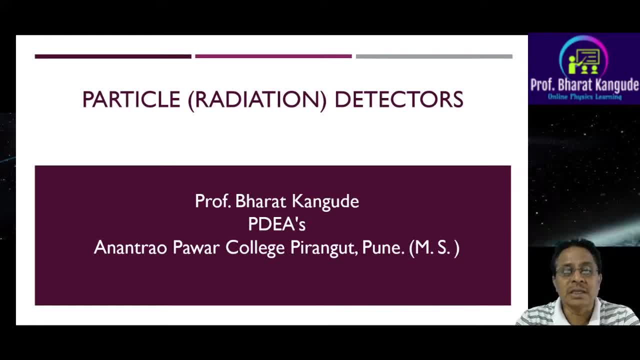 us in any nuclear reaction or in nuclear physics, to understand what are the particles that are we are coming in contact with, because these detectors play a very vital role whenever there are certain radiations or some certain radiation accident happens And in that case, whether that particular area or that particular installation is safe for humans or not. that 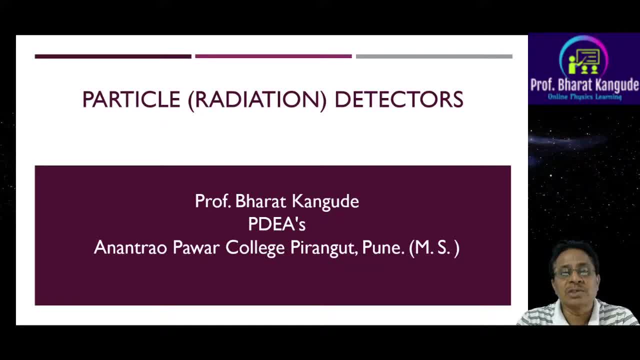 is to be tested, either for alpha, beta, gamma type of radiations or some other radiations. radiations are thus much hazardous for human if a proper protection is not taken or if a proper care is not taken. sometimes this radiation causes a lot many physical problems and in such cases 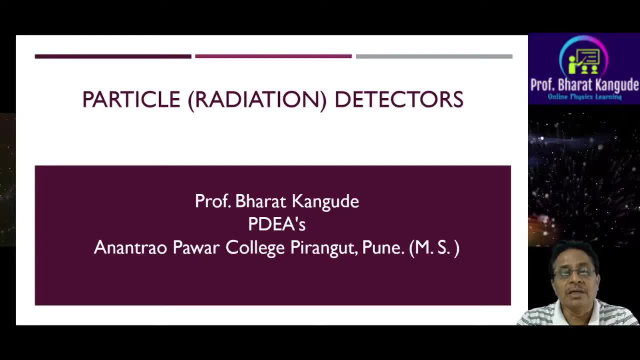 of accidents or somewhere, we require certain devices that will detect that presence of the radiations. as we have seen, there are several different types of devices in in medical physics we use where such type of radiations are generated and these radiations, so their safety level, is to. 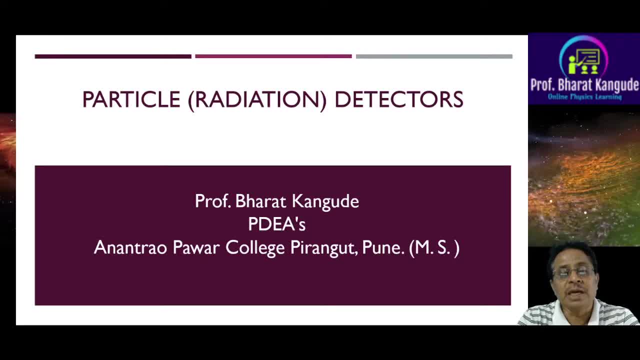 be maintained and to maintain this type of safety level again, we require certain types of devices. now, what are these devices? how to construct them, what are their properties, what are their other types of aspects that all these things we are going to discuss in here for the discussions? 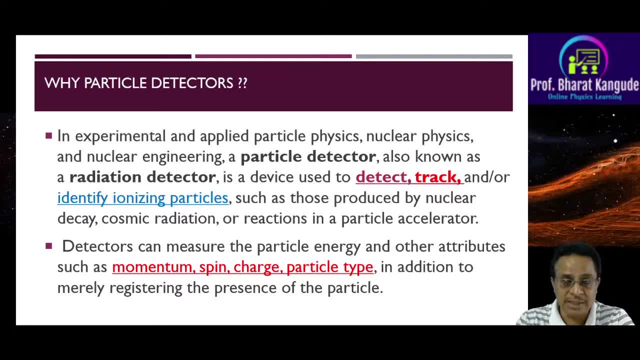 so, as we have discussed, why particle detectors? why they are needed, what is the use, why? why? what will happen if we don't protect them with the radiation that we will be using? have such type of particle? don't have such type of particle detectors. these are the few questions. 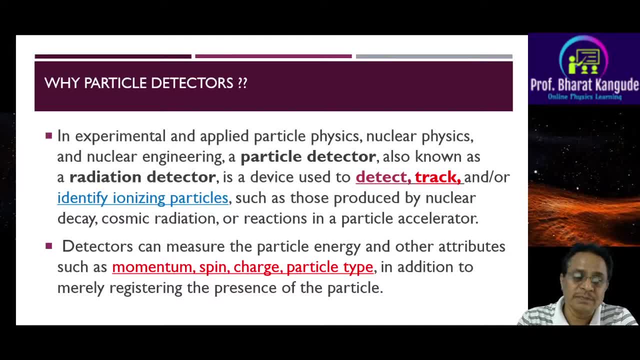 we have to answer first. so why particle detectors? in experimental and applied particle physics, nuclear physics and nuclear engineering engineering means the nuclear reactor engineering, if of course it is a particle detector also known as a radiation detector, so both of the names are just same. particle detector, or you can call it to be a radiation detector, is a device used to 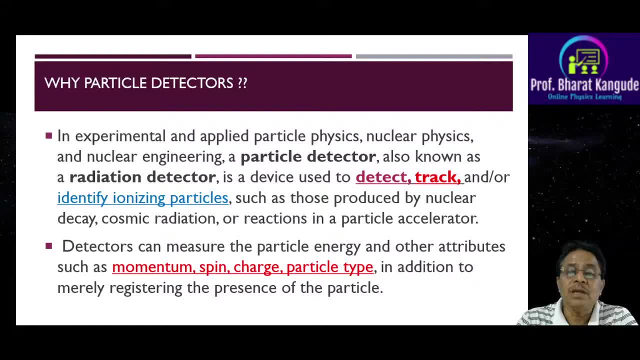 now there are the four functions: track, detect, track and or identifying ionizing particles, such as those produced by nuclear decays, cosmic radiations or reactions in a particular accelerator. so whatever type of nuclear reactions going around us, whatever type of nuclear decays going around us, whatever type of nuclear decays going around us, whatever type. 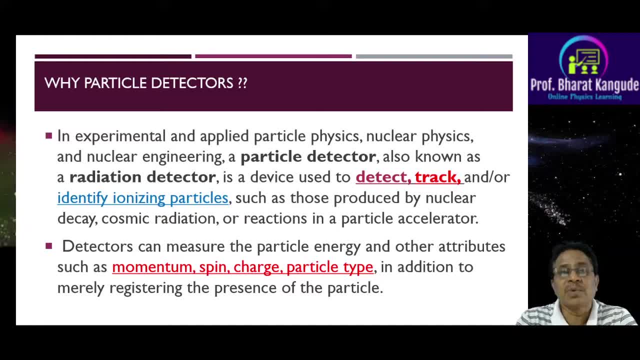 of number of particles that are ejected in that process. these particles are to be detected first. then we have to track their journey from their path to, and we have to identify whether they are ionizing the material medium around them or some such type of any effects are observed or not. 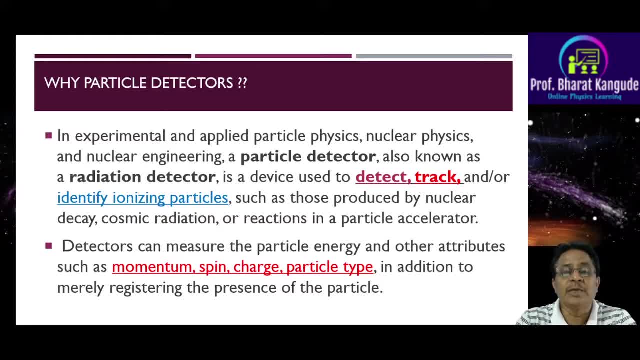 all these things are to be tested, are to be detected, are to be tracked, and this is what the major application of all types of particle detectors now here, second paragraph: detectors can measure the particles, energy. some detectors, we directly measure particles, energy and other attributes such as: sometimes we are able to find out their momentum of the incident particle or the 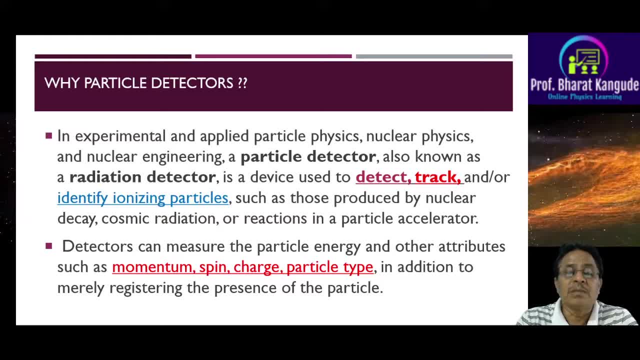 outgoing particle, the spin, the charge, particle types, etc. depending upon the device we have selected, depending upon the device we have designed and using. based upon that, several other parameters of such type of particles, which are emitted in different types of nuclear reactions, can be identified, can be measured, in addition to merely registering the presence of the particle. 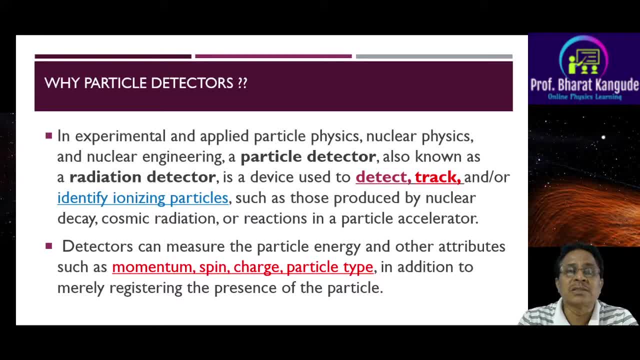 So some devices which directly tells you that such and such radiations are present in that particular region or in that particular area. Some devices directly specifies what these particles are, what are their energies, what are their other parameters, like spin, charge, their type, etc. 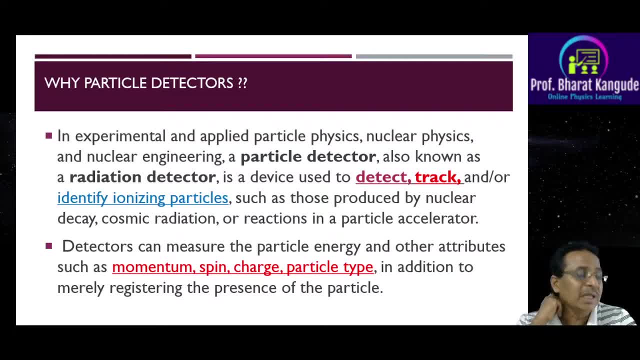 All these types of things can be decided and can be studied with help of these devices, which is called as particle detectors. So, as we have seen, accelerators are very important tools of this type of nuclear technology. Detectors is also one of the very, very important tool of this nuclear 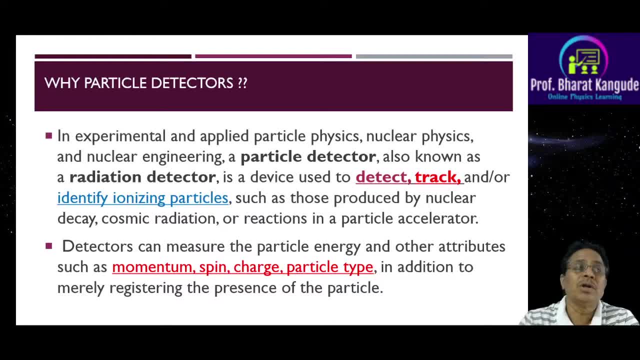 technology. Please note, without detectors it would not have been possible for any nuclear scientist to identify the particles, To study the radiations, to study the radiations and to study this type, different types of nuclear reactions which we are rightly seeing right from the beginning. So these detectors plays a very 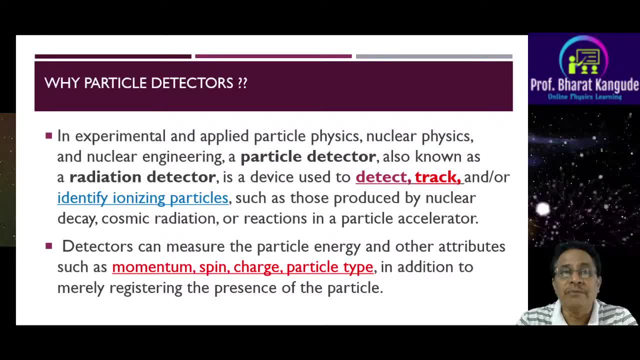 very vital role in the development of the nuclear physics itself, as well as nuclear technology. Thereby we can identify different particles, we can see their properties, we can understand the properties, we can understand such type of physical phenomenon. In that sense these tools, detectors, are. 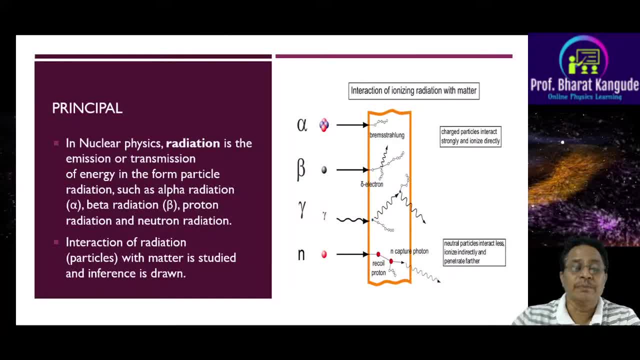 very important Tools of the nuclear engineering. Now, what is the basic principle used by all such detectors? that can be seen in the following slide. So in nuclear physics, radiation is the emission or transmission of energy in the form of different types of radiations. Already we have called them. 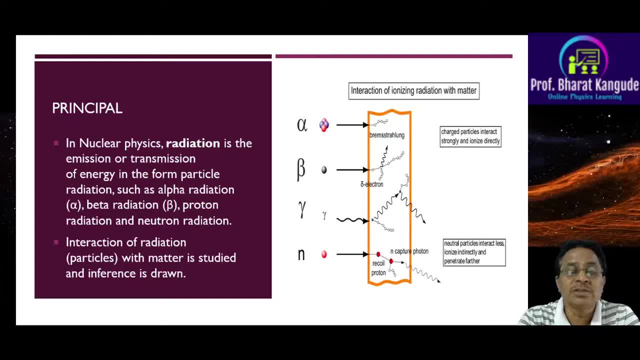 alpha, beta, gamma radiations, sometimes neutron radiation, sometimes proton radiations and so many things, Beta plus, beta minus, etc. And there is always an interaction of radiation, of the particles, charged particles- with matter which is to be studied and inference is to be drawn. That means studying the interaction of this type of particles emitted in 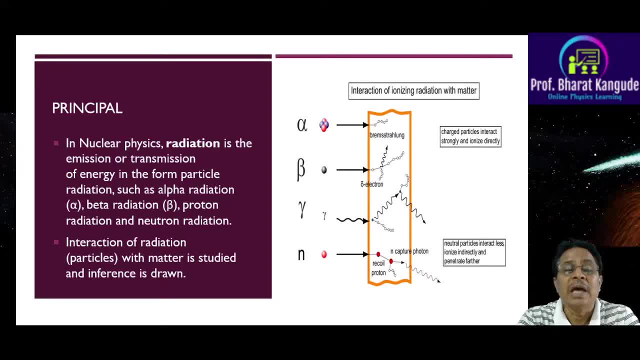 such type of nuclear reactions with matter and analyzing this behavior of this particles, That is what we have to go for certain inference and we have to identify that particles, We have to infer their properties, We have to see what has actually happened in this type of nuclear reaction. 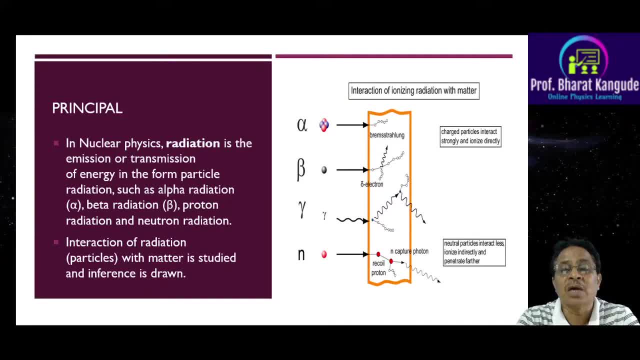 For that. these four different approaches have been shown there. Right hand side shows you interaction of ionizing radiation with matter. So this is matter, sorry, radiation matter interaction or energy matter interaction. In fact, in physics you might have learned several different types of interactions, For example, if there is a mirror and some light falls on that mirror. So this is. 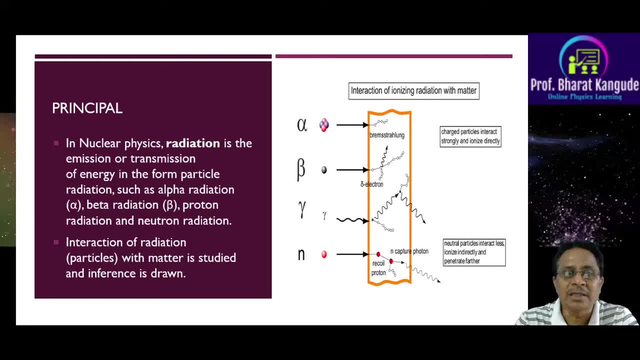 light and matter interaction too. So this is an electromagnetic interaction Here in the nuclear physics. whenever these type of particles ejected in the process, either alpha, beta, gamma, neutron or proton, These particles interact with materials in different manners, as shown in this particular diagram. Some particles are charged one, Some particles are. 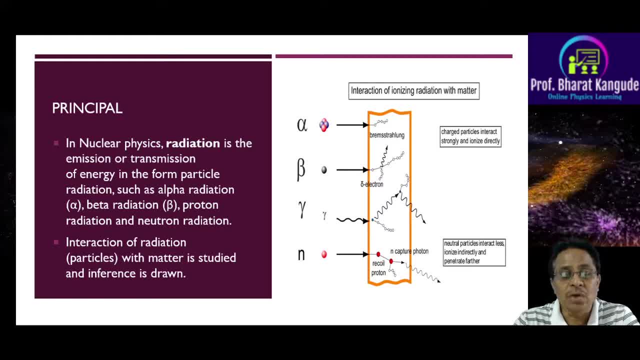 neutral. Neutral in the sense gamma has no charge, Neutron also does not have any charge, So it's a neutral, Whereas alpha, beta and proton. these are the charged particles. Now behavior of charged particles in certain materials and behavior of uncharged or neutral. 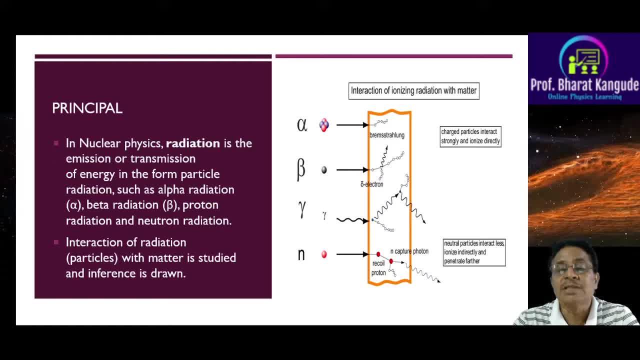 particle in certain behaviors, certain materials. These are the two different things we have to understand at the beginning. So now let's see the first part. The charged particle interacts strongly and ionize directly. So that is direct ionization of material medium and the strong interaction. 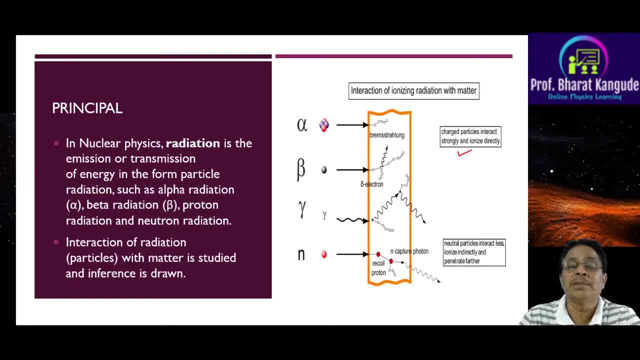 between these type of particles- incident particles- and that material happens. So this is shown to be a material Initially. when this material is ionized, the ionization of the material is done. Alpha particle incident upon this material. There is one very interesting process that is. 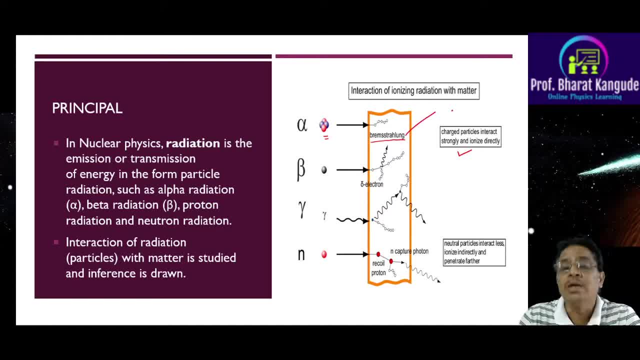 called as bremsstrahlung. It's a German word. Bremstrahlung means breaking radiations. So when, whenever such type of particles interact with the matter, this particle loses energy in a very small time. and whenever it loses energy, this energy comes out in the form of. 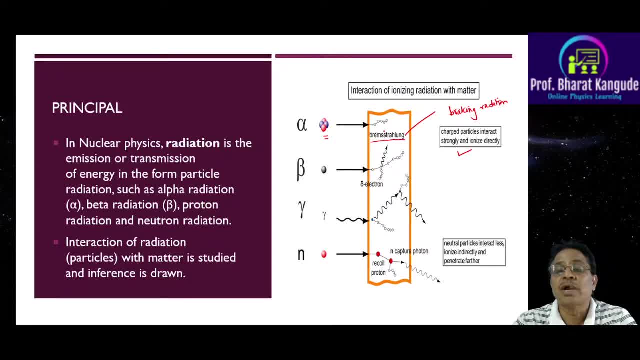 electromagnetic radiations. So this process is called as bremsstrahlung. So in case of alpha particles and beta particles this phenomenon of bremsstrahlung is observed. Only thing here: it is shown that this, the penetration range or the penetration power of alpha particle, is shown to. 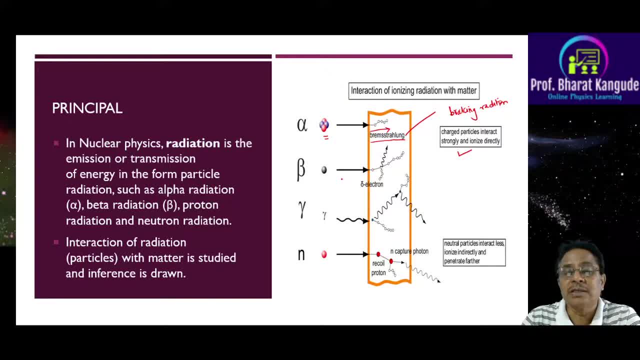 be somewhat less, Whereas for beta particles or this like electrons, this range is little more. So this penetration power of beta particles, or this beta radiations, is more as compared to alpha radiations. Here also the process of bremsstrahlung is there. Sometimes this beta particles dislocate. 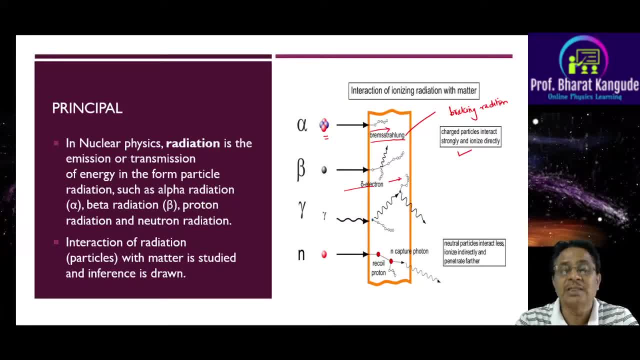 the internal electrons of that atoms inside this particular material medium, and further processes are also possible, and this particular processes are seen here Now. these interactions are very, very important and basis upon this interaction, we infer that incident particle is either alpha or beta or something else. That is what this is, what interaction of charged. 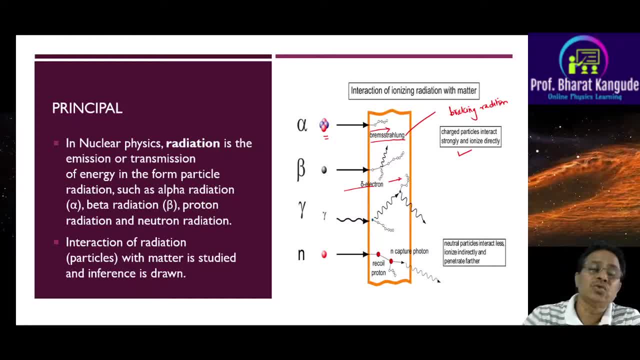 particles with these certain materials. On the other hand, these are the two particles, gamma radiations or photons. when they incident upon the material, Then this gamma particle also uses its energy and it gives energy to electrons inside. So such type of effect effects already. we. 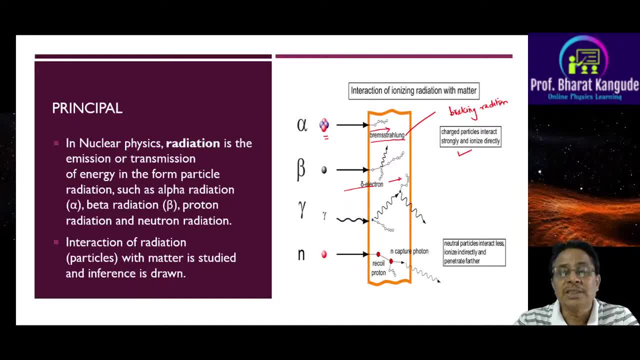 have seen in photoelectric effect. Electrons are emitted from the internal structure of this atom and such type of effects are called as photoelectric effects. So this is one more interaction. We are using these two in some of the instruments. that's why we are studying it here. 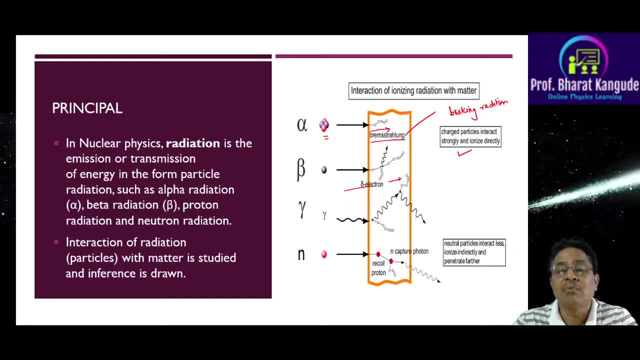 These type of interactions are also possible where their type of photoelectric effect is observed. Sometimes there's a neutron which is neutral and this type of neutrons, when interact with this material medium, some of the neutrons get captured by the nucleus or nucleus of that material medium. 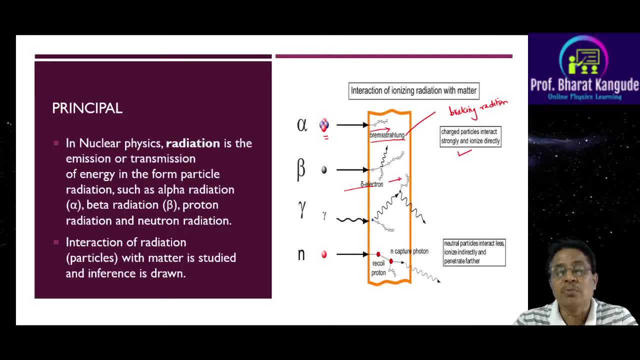 easily captures this neutron. There are several different types of phenomenon associated. that is called as nuclear reaction, cross section and all these things which you have not learned here. But there are several reactions in which of the nuclei in which there are neutron and they easily absorb this neutron, and that type of reactions are called as neutron capture. 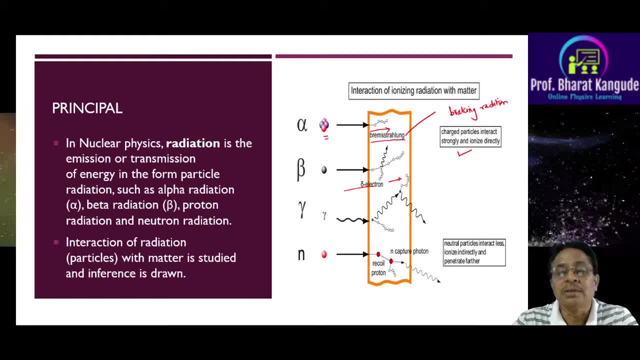 So either bremsstrahlen or photoelectric effect, this neutron capture, etc. these are the different phenomena with which this radiation interact with this material medium. Now, material medium can be solid, can be liquid, sometimes gases, sometimes vapor. depending upon different types of device, these material mediums may be of different nature. The second, the the last, last two. 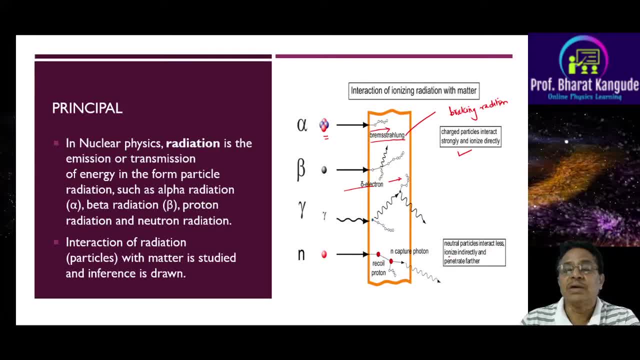 here it shows, the neutral particles interact less, ionize indirectly and penetrate further. So penetration power of both of this is very high. Already we have discussed in this particular chapter number two, that is, radioactivity. This gamma radiations have highest penetration power because they interact weakly with the material medium particles. that's why they travel more. 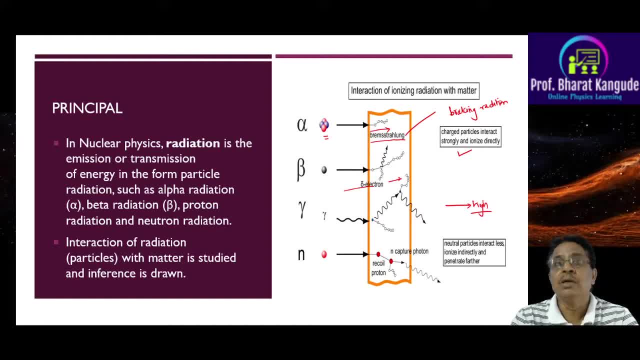 inside this material medium. that's why they have higher penetration, lowest ionization. On the other hand, alpha particle has lowest penetration, minimum penetration, but it has highest ionization power. So, depending upon this type of different types of phenomenon, natural phenomenon occurring between radiations and matter or material medium, we can classify, we can identify, we can study, we can. 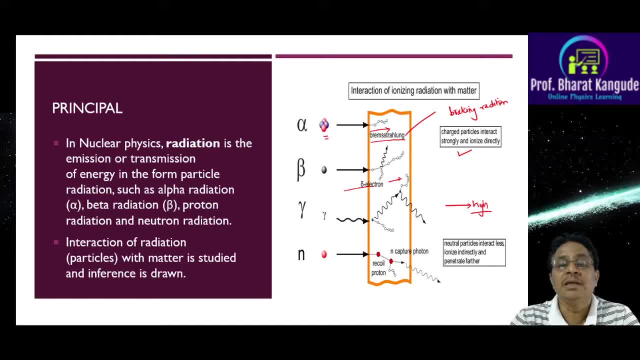 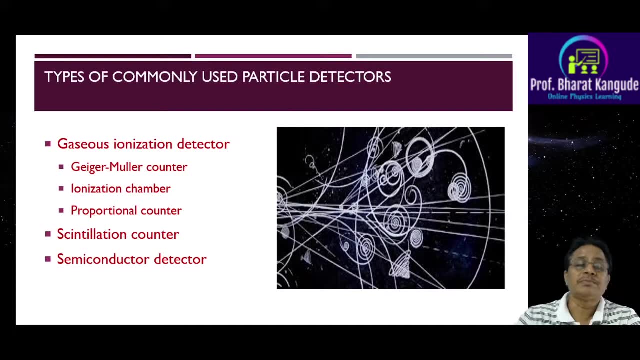 infer the properties of different types of particles and the interactions nuclear reactions vary in such type of particles are emitted. So henceforth, in all of the devices we are going to use, at least one of the principle, what we have seen here, That's what the another important point. Now let's come to the types of commonly used particle. 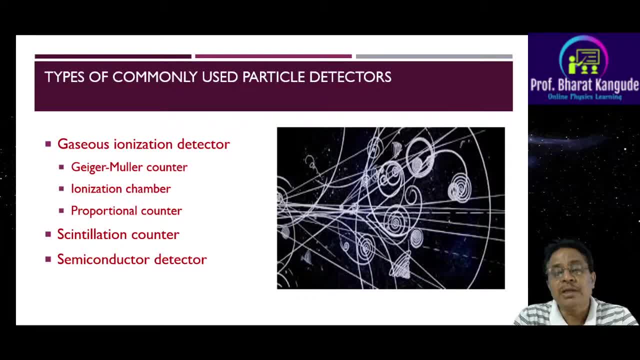 detectors. I have shown one such diagram to you. In that particular diagram, these are shown to be parts of the different particles that have been followed in certain chamber. Actually, this is called as cloud chamber. This is what is a cloud chamber. There is some. 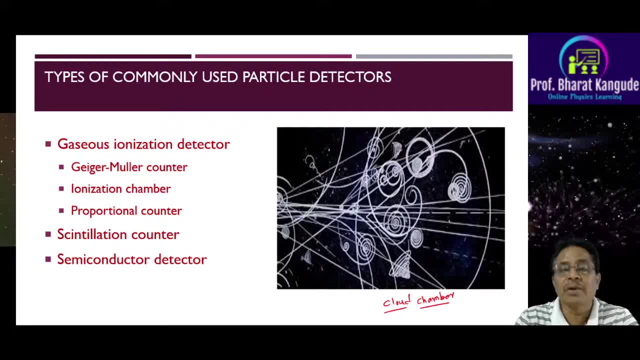 that that is called as the saturated vapor of certain materials is placed in this chamber Whenever particles do follow. Now see this: there are certain particles which are going directly in a straight line. There are few particles which are going in a curved path. There are few particles which are emitted in this process. So here some reactions takes place. 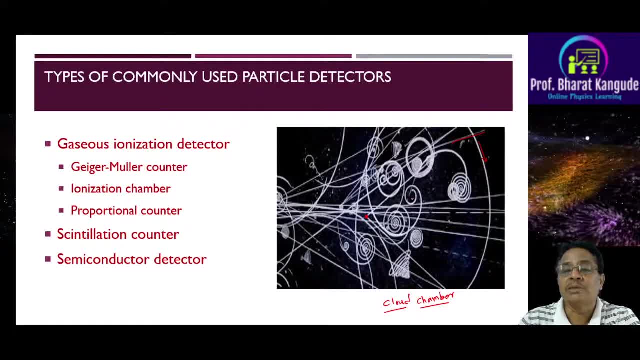 and this particle now goes, is here and then starts revolving like this. So these are the two particles which has gone here. There is another particle which has gone here. Maybe these are antiparticles of each other. because of their directions We can infer that. 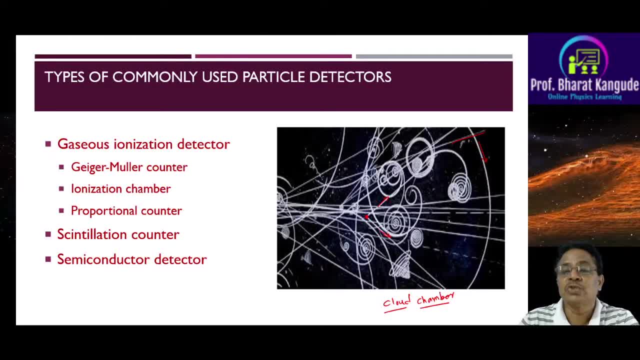 these are the two antiparticles. There are some other particles which are showing to be a spiral, as shown by this, and then this particle automatically finish. So this complex picture is the photograph taken from a cloud chamber where certain particles are allowed to interact with this. 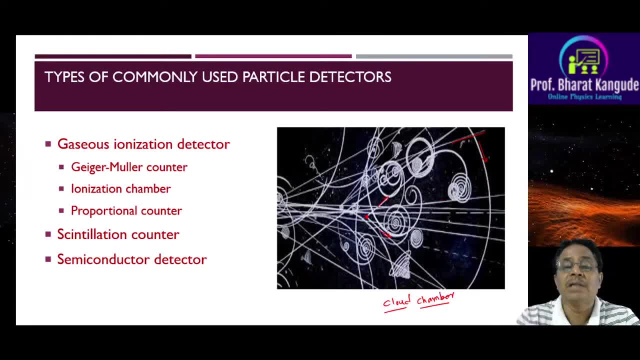 material medium. Depending upon the situation, different particles follow different paths And studying this nature of the path we can understand properties of that type of particles. So in that sense there are three different types of materials, or three types of the commonly used particle detectors are there. So first one is called as gaseous ionization detector. 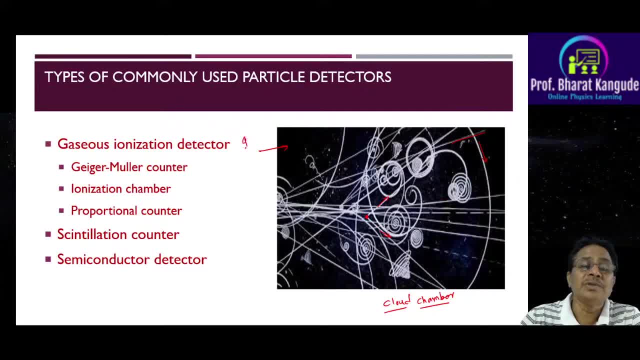 So this is the gaseous ionization detector. Gas medium is used here, basically for ionization purpose. and looking at this ionization path, or these paths of which this particular particles have created, Studying these paths, we can understand properties of some of the 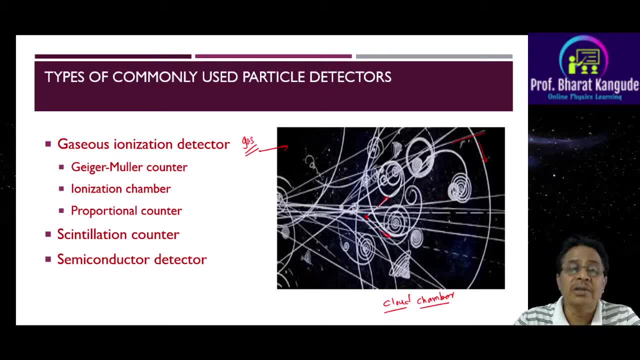 particles, So the detectors which are using gases for ionization process. these are called as gas ionization detectors. Very common and important among this is GM counter or Geiger-Muller counter, which we are going to discuss in detail. Then there is some ionization chamber which we have. 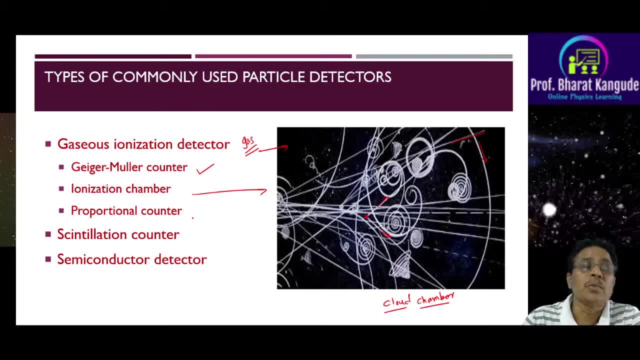 been shown here. This is one ionization chamber. There are certain proportional counters too. Then there is a second type that is called as scintillator counter. That example of that also we are going to discuss. These are the certain solid materials are used. 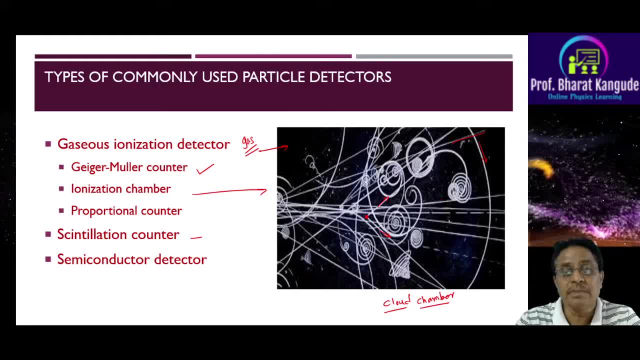 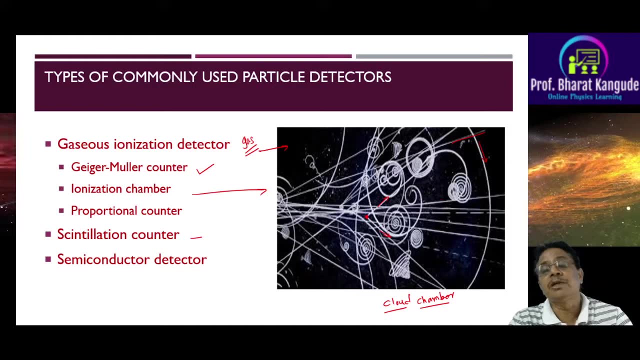 in this case, and phenomenon of interaction of energy with matter. That is very nicely used in this case to count or to detect such type of incidence of the particles. Then in some of the detectors, semiconductor materials are also used, And studying the properties of this semiconductor. 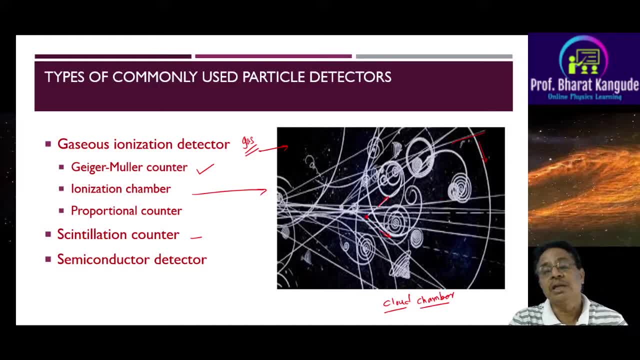 materials. when such type of particles incident, we can understand their behavior too. Apart from that, there are several other types of ionization detectors which we are going to discuss. So there are several other types. May be 50-60 different types of detectors are there. 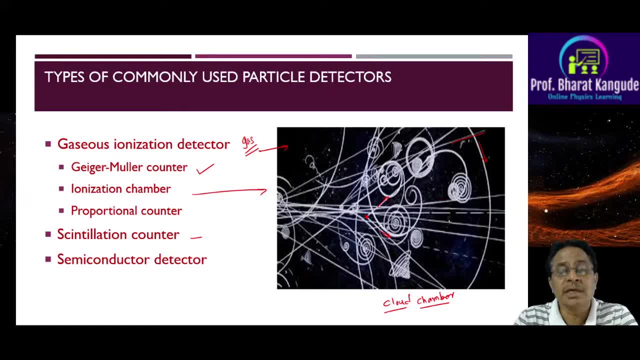 As this technology is advancing, more and more advanced detectors are coming in, Nowadays very hand-fold or easy to handle, easy to operate. such type of detectors are there, available in market And some of the easy operators we are going to understand or we are going to discuss here in the following. So there may be list, may be very, very large. 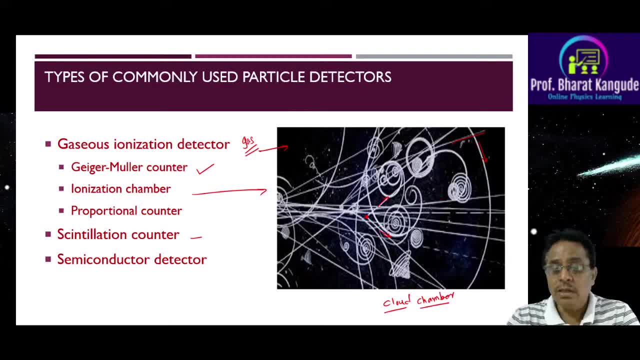 10,, 20, 50 number of different types of particle detectors are there. Out of that, we are just going to see these two. first one is called as GM counter, Geiger combined counter, and second is called as skin collision counter. So these counters directly measure the number of particles. incident. 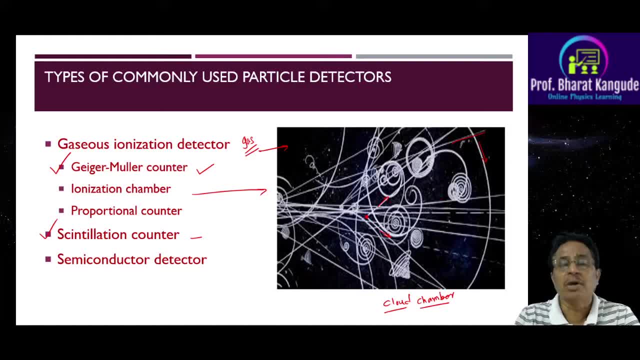 per unit, second, near minute, per hour or per day, etc. So we are just counting the number of particles which are incident upon this material Or these are emitted by a particular source. Reductive source may be alpha particles, beta or gamma particles. So in that sense we haveρί. 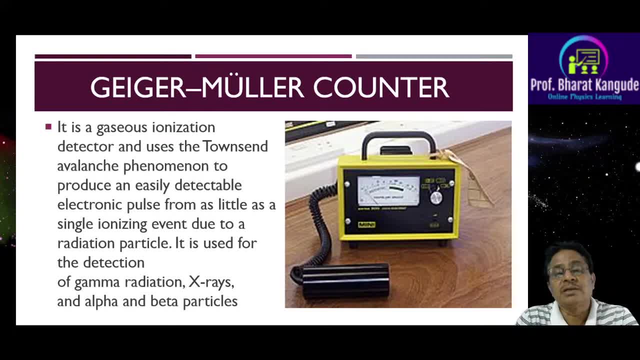 in that sense. let's see the first one that is called as Geiger-Muller counter. so see this. these are the. both of these scientists were german scientists who invented for the first time such type of detector, and here this is the basic device. okay, so diagram has been shown here. 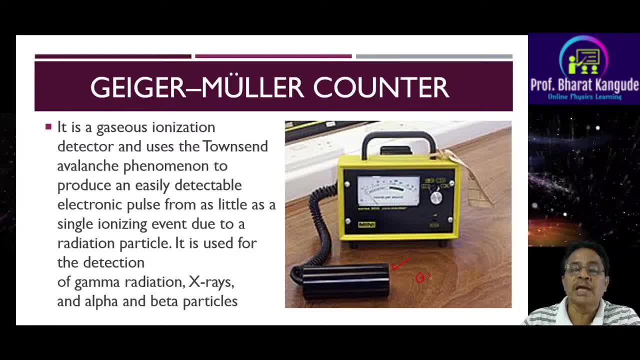 this is the device where this type of gm tube- so this is the actual gm tube and this is all other okay accessories here- where there is a meter, there is a cable connection, all the circuitry inside that we can change its ranges, we can make it on or off and etc. and this particular assembly is 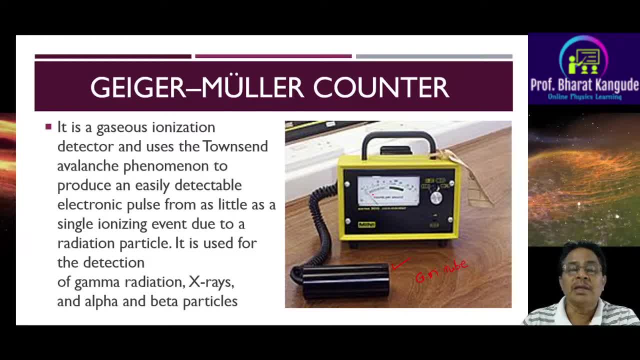 associated or disconnected to this gm2 and thereby number of particles or the current generated by such type of interaction. that is recorded here and this becomes a gm counter. so this is one type of gm counter which has been shown here. out of that, this black part or this black type of pipe or type, 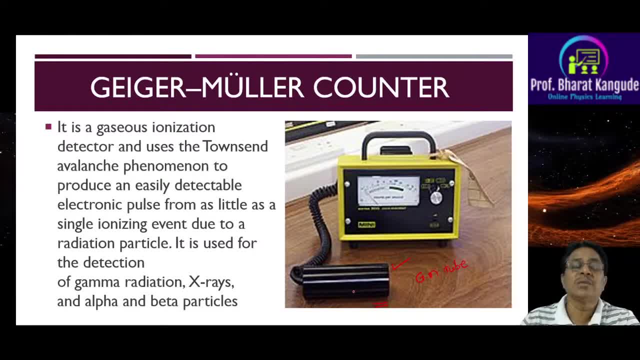 of part shown here. this is actual gm2, where this type of interaction takes place. so this particular thing reads as this: it is a gaseous ionization detector and uses- this is one phenomenon called as Townshend avalanche phenomenon- to produce an easily detectable electronic pulse. pulse is 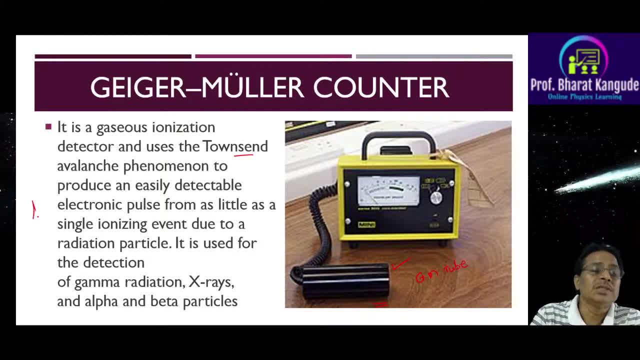 generated. okay, so when one particle comes, one such pulse is generated. when other particles come, another pulse is generated. so such type of pulse are generated and these pulses can be counted by this counter and depending upon that we can count very easily how many such particles have been. 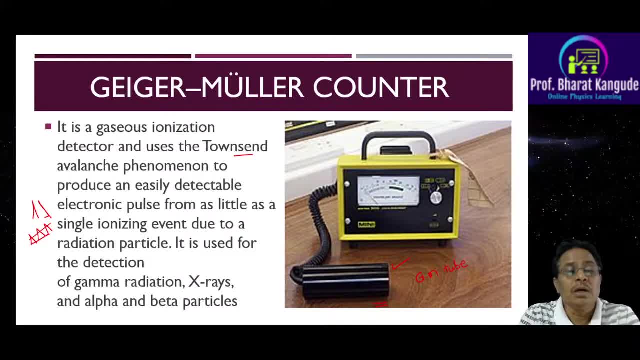 incident there. so phenomenon to produce an illicit, easily detectable electronic pulse from as little as a single ionizing event due to a radiation particle. that means single particle is coming and because of that a small electric pulse is generated and counting this pulse we can identify presence of such type of particles. and this, this gm counter, is usually used for detection. 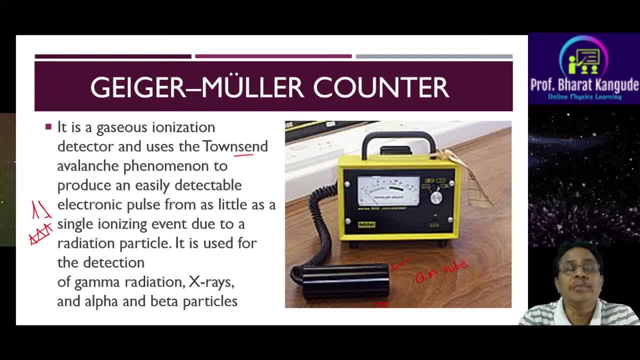 of gamma radiations, x-rays, alpha and beta particles. so for gamma, for proton, etc. this type of this particular type of device is not usually measured used. so gamma radiations, gamma particles, x-ray radiations, alpha particles and beta particles, these are the elementary particles which are 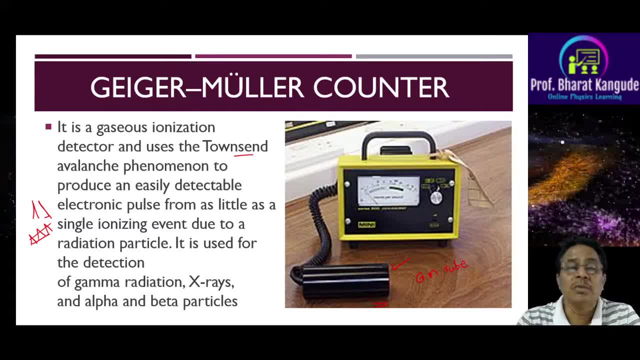 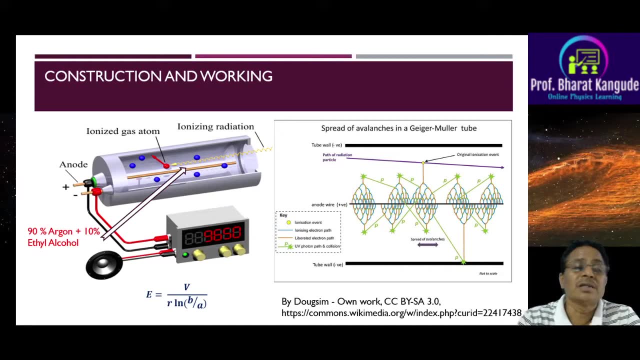 usually measured using this gm counter or geiger-muller counter. now, in sport, we are going to describe its construction. we are going to describe in brief, it's working. then some other characteristics of this type of devices that will be discussed as follows. let's start with this now. this is a construction and working. so these two 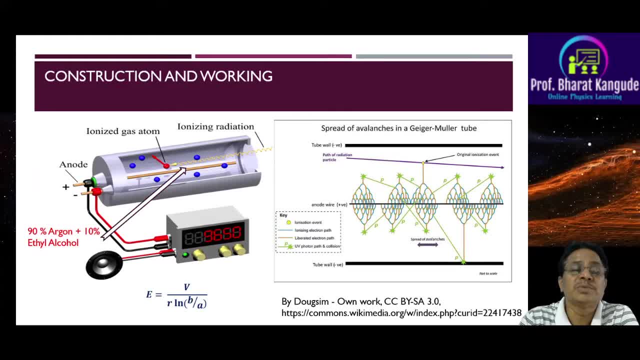 diagrams that show you what is the construction and how this particular gm counter functions. so what is the actual phenomenon that is occurring that's shown here. so that shows you. this is one tube that is called as anode tube, which is made up, sorry, diacathode tube, which is made of certain. 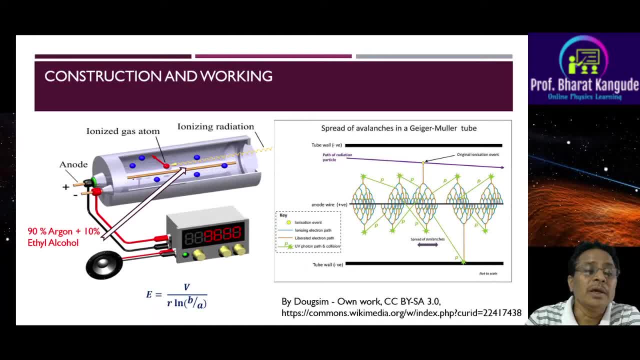 material and cross section of that has been shown in. in the okay center to this particular tube there is one thin wire which is called as anode and which is connected to this positive of the battery and this cathode which is connected to negative of this battery. so this is source. 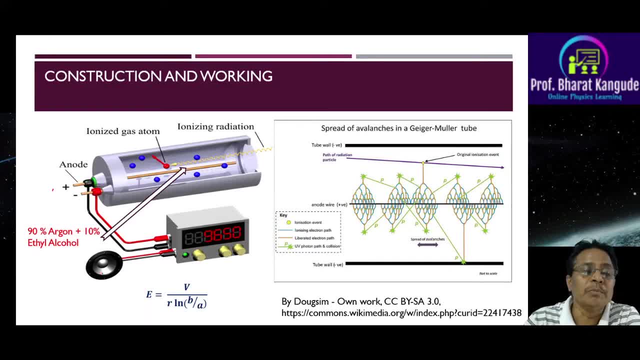 and recorder 2, which is connected to this particular buzzer again, which gives a buzzer whenever this type of radiation incident occurs. now, here, in this case, you will find that inside this tube there is a mixture of 90 percent argon- argon is a in non-reactive gas- and 10 percent ethyl alcohol. so this mixture of this material, 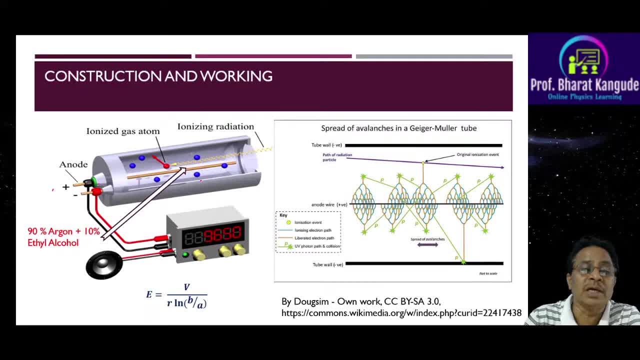 medium is used inside this, which is shown by these blue dots there, and whenever a incident radiation comes here, which is shown here, this is ionizing radiation which is coming in from this window. so this is a side from where this type of particle and this is called as window of this tube, and when this particle interacts or come inside this. 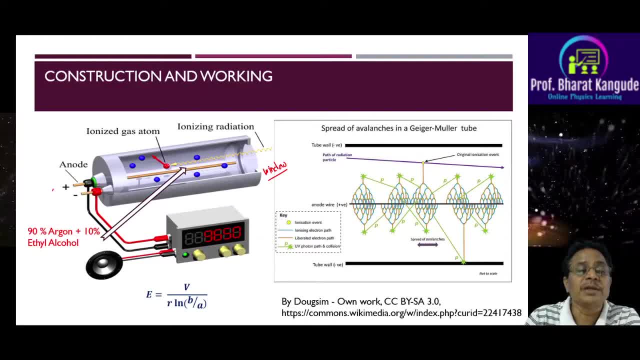 material medium here. in this case, this particle interacts with this molecules or atoms of this type of material medium, and that is interaction- gives rise to a phenomenon that is called as, as what we are going to discuss here, secondary electrons are generated. these electrons are so energetic, highly energetic, because in this case potential used is very, very large, almost around 1. 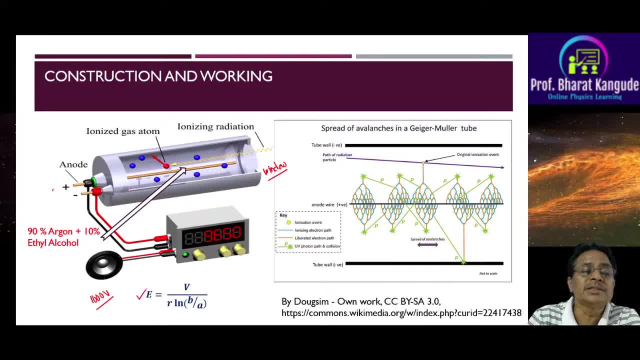 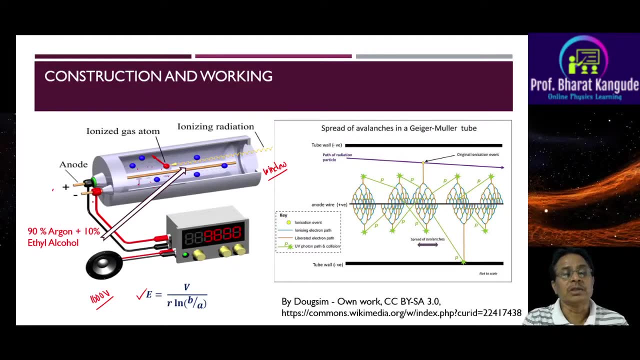 000 volts and large electric field is generated inside this, at different points of this particular tube, around this particular anode, which is given by capital e is equal to capital v upon r. r is the radius of this particular uh anode, of this particular anode wire, then uh, this r is the distance at which that means from this anode wire. 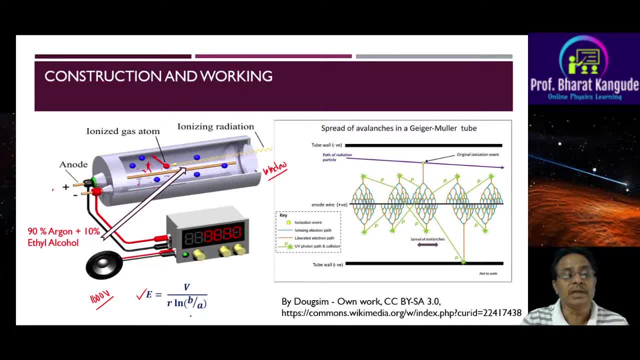 at what distance we are supposed to find out the value of this electric field there. this is: V is the potential applied across this anode and cathode and this is ln log of natural log of B. B is the diameter or the radius of this particular tube itself and small a is the radius. 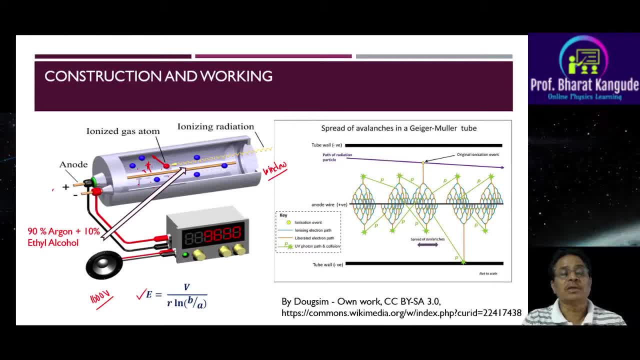 of that particular anode wire. So anode wire diameter, the tube diameter ratio of these two has to be taken log of that and multiplied by R. So this expression gives you value of the electric field at any location at a radial distance, R away from that particular anode. So this is an 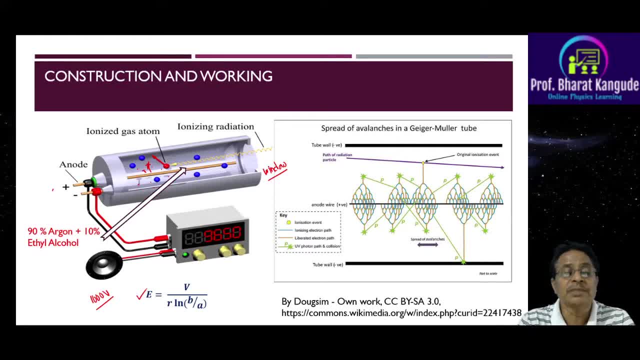 expression which directly we use directly in the electrostatics, and this relation gives you electric field produced inside that. So whenever such type of incident particle comes in. So second diagram shows you. this is what a cross section has been shown. This is a tube wall. This part is shown. 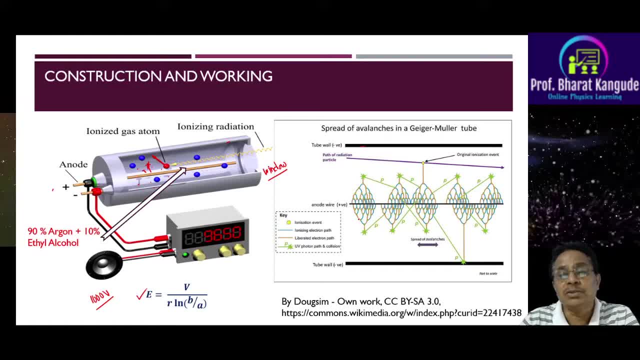 here. This is tube wall In between. this is two sides of tube wall. This is what anode wire, which is necessarily anode wire, This is anode wire, This is anode wire, which is necessarily anode wire. positive, kept at a very high potential, around 1000 volts. as compared to this anode Anode is almost. 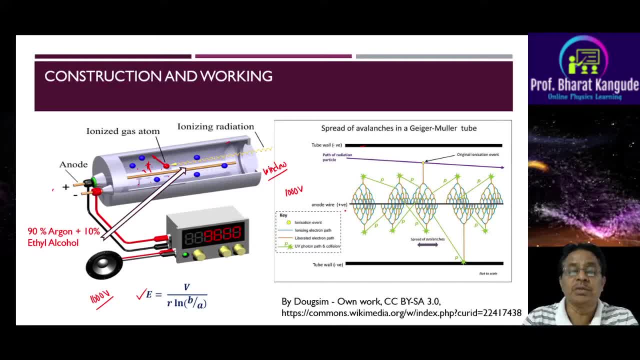 zero volt and this positive recharge, positive side of the batteries to be connected to this anode, which is having its voltage in the range of more than 400, 600, 500 or 1000 volts, and so on. Now, when this incident particle comes here, that shows: 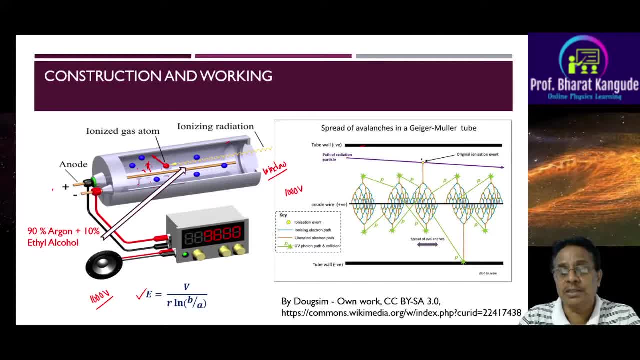 it interacts with the incident particle. This is this molecule, like argon and like that, And in that process, this particular, there is interaction between this radiation and this particle that produces this type of electron. So this diagram shows you. this is an ionization event. 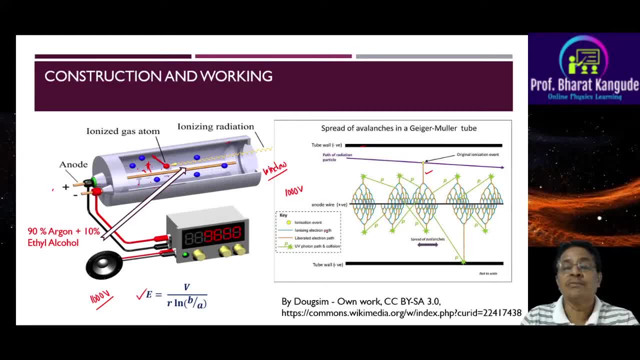 Then this is the ionizing electron path. So electron which is ionizing further metal medium molecules, that is shown by this blue color, Whereas liberated electron path, electron which is liberated in the process, that is shown by this brown here and this P symbol, P UV photon path. 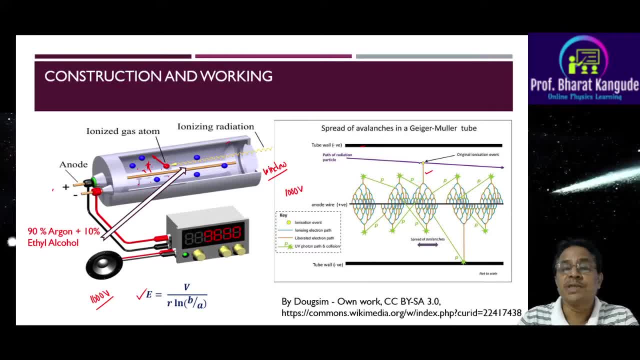 and collision. So whenever such type of incident particle interacts with this material medium, this type of electrons are liberated and since electron has negative charge, this anode is highly positively charged body. This accelerate these electrons very heavily and in that acceleration this electron gains a lot of amount of energy and this undergo for further process of this. 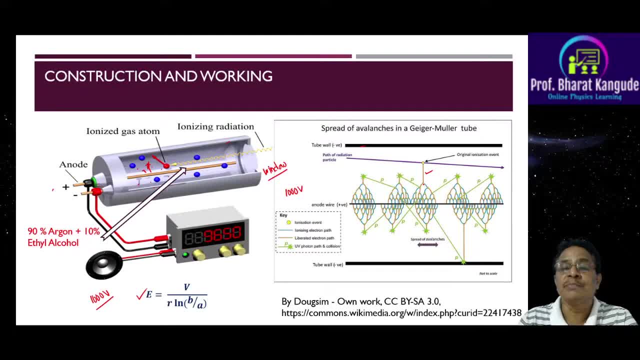 ionization. So here also another ionization takes place, And in that ionization one more electron is generated, and another electron here that is found to be ionizing path. So this is another electron. So from this, so this particular shows you, when a single particle is incident, single radiation is incident, it produces this electron. 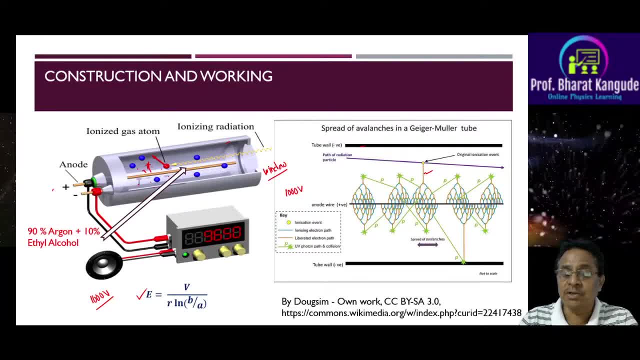 and in the journey from now. this is an, this is a. electron is a negative charge particle, and that means ion and electron pair is generated, Electron being negatively charged. this gets attracted toward this anode, Whereas this ions that are produced because of this charge- negative charge, sorry, positive charge- they get attracted toward this anode. Anode is negative. 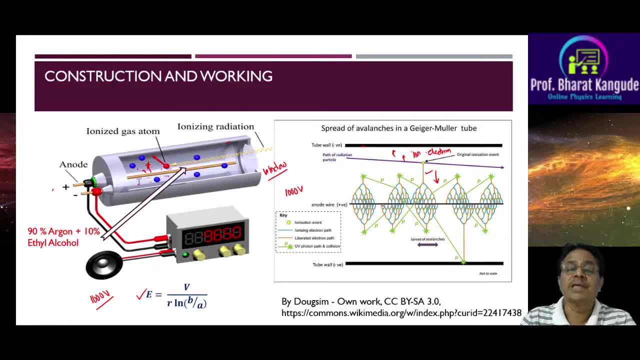 as compared to sorry- cathode. Cathode is negative as compared to anode to certain extent. So there is a movement, clear cut movement. ion goes this direction, whereas electron goes in this direction. Now, because ions are bit heavier as compared to electrons, the speed of the ions going 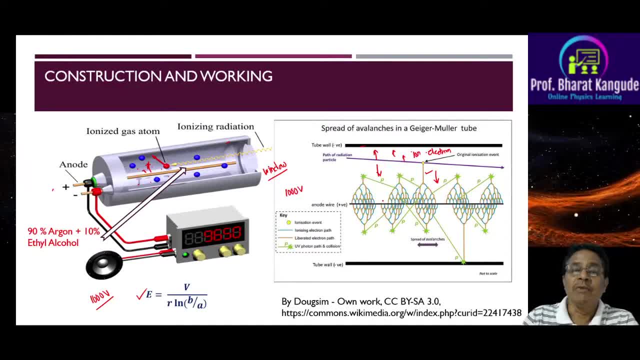 this location to this cathode is very less, Whereas this pair speed of the electron that are attracted toward this anode is very, very high. In that process, these electrons interact with other types of molecules or atoms and they produce this secondary electrons too, And large number of such secondary electrons are generated after a single particle incident. 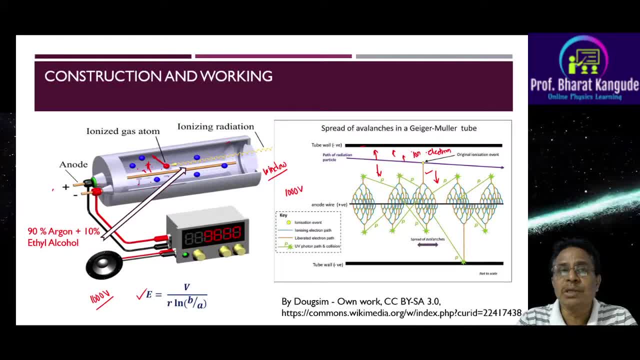 and, depending upon that, a that is called as a pulse is generated: Large number of electrons, time that arrive on this anode, and this anode is further connected to certain load and that gives you certain current through this anode, and a current pulse is generated in this case, So that 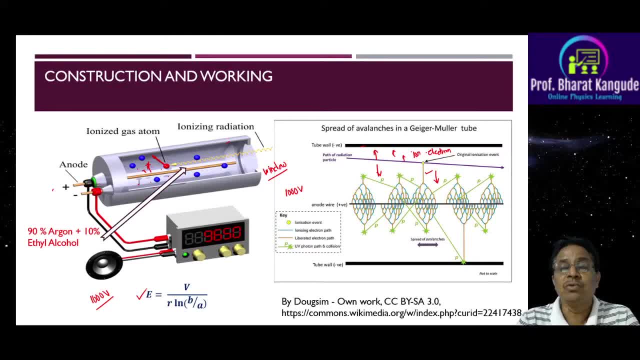 is how- this is what the working of this type of gm counter that takes place- that incident particle that ionizes the material medium, Ion and electron is created. Electron gets accelerated towards the anode because it's a positively charged wire which accelerate this electron very heavily. 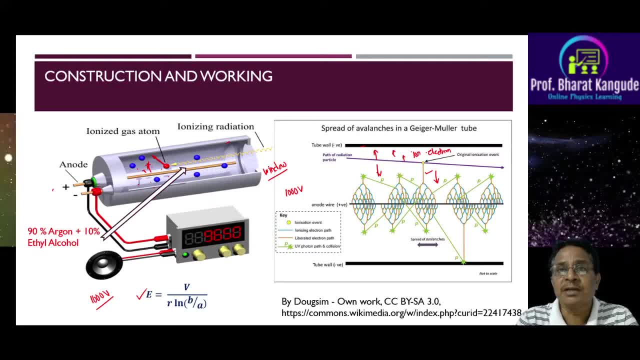 in that process, this electron gains energy and secondary, tertiary, fourth time electrons are produced. A large number of electrons are produced due to a single such type of incident- particle- and this is called as a Townshend avalanche. Avalanche means large number of electrons are. 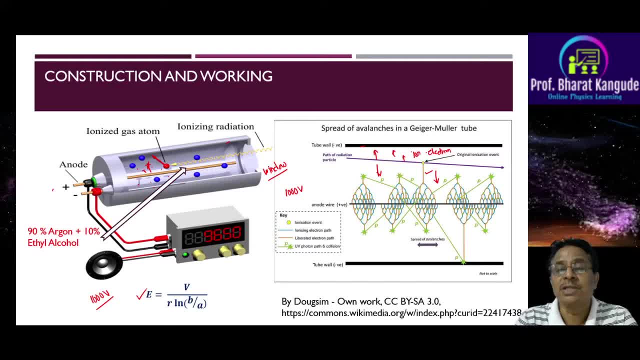 coming simultaneously and that causes a creation or generation of a pulse, Whereas the ions that are generated, which are basically a positive ions, these ions are accelerated toward this tube, well, tube wall, or the wall of this particular tube, But in this process, as we see the speed of 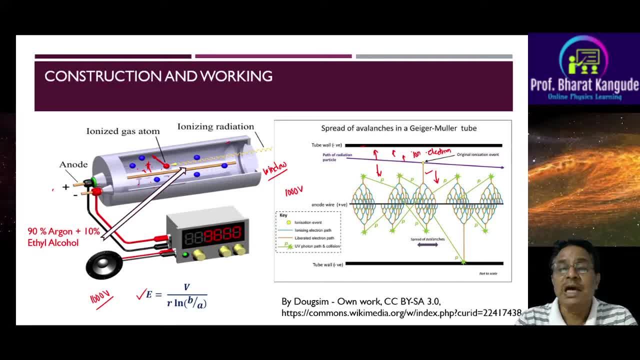 that is always less because of their heavy masses and this particular thing. that means whenever an incident particle comes, such type of pulse is shown by this device. These pulse are recorded and per minute, per second, how many such type of pulses are occurred there? This is to be measured. 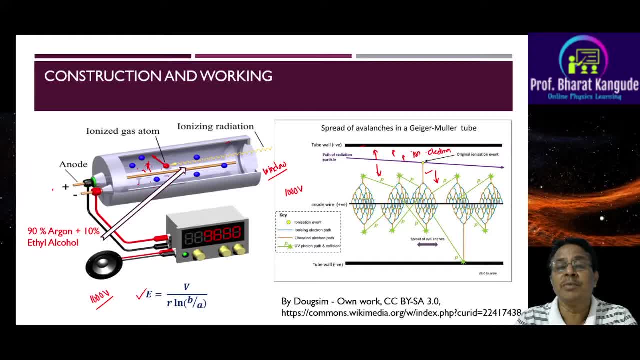 and based upon that we measure the incident particle, How many number of such particles incident that is counted by this particle. So this slide is very important, slide that tells you what is actual functioning of that particular device occurs and what is the phenomenon that actually occurs here. Now, this particular 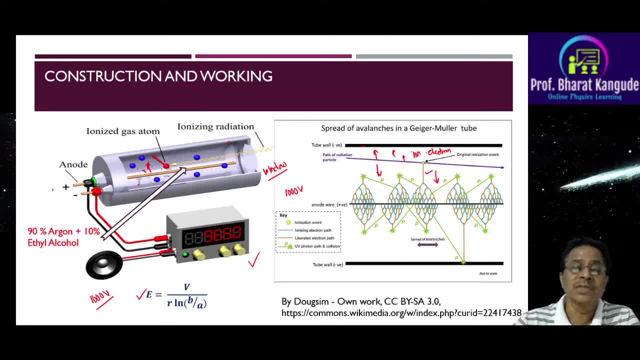 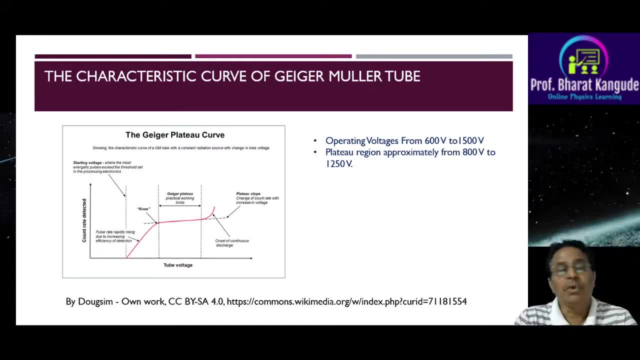 avalanche is called as Townshend avalanche, which gives rise to a certain electric pulse immediately when this incident particle appears there. Now, in that concern, we have to go for certain characteristics for GM counter or GM tube. This characteristic curve is very interesting. curve Now see. this curve is very interesting. curve Now see. this curve is very interesting. curve Now see. 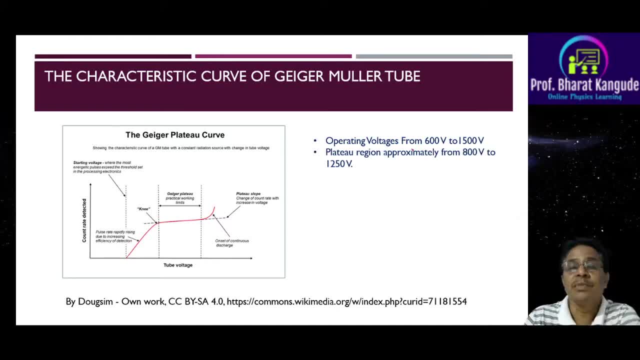 this voltage. Voltage is range in this operating voltage for any any such type of GM counter is almost 600 to 1500 volts. This is the range. So below certain voltage there is no count observed, even though particles are coming, if this type of voltage is very, very low between anode and cathode. 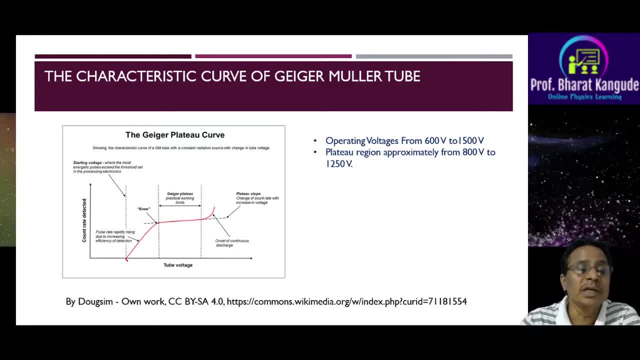 then this type of reactions, of this type of interaction, usually doesn't happen. that means there is no gas discharge. Since there is no gas discharge, there is no electrons will be produced. Secondary or tertiary electrons will be produced and therefore that particular signal generated will be not there. So to have such type of effect occurring inside this tube, we require certain 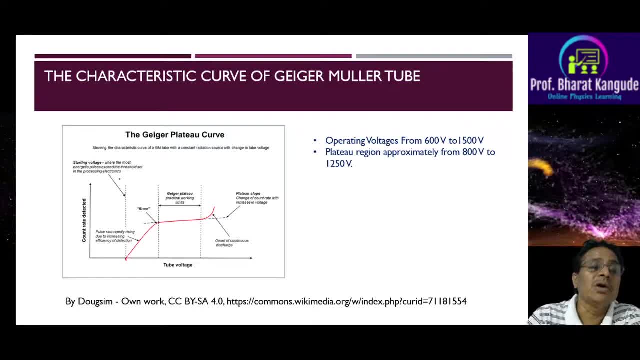 minimum type of potential that is either called as starting voltage or it is also called as threshold voltage. Then it is observed This is usually around 600 volts. Then when this particular we start this increasing the voltage, now more and more number of particles are incident. These 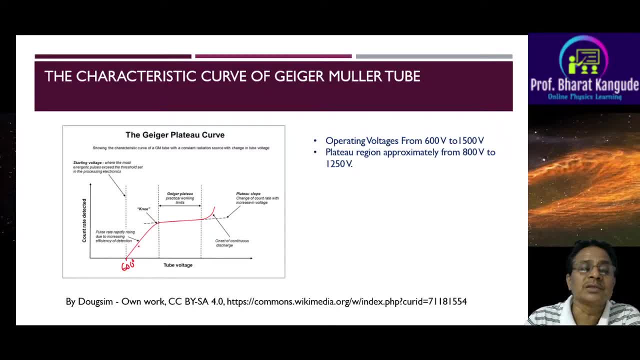 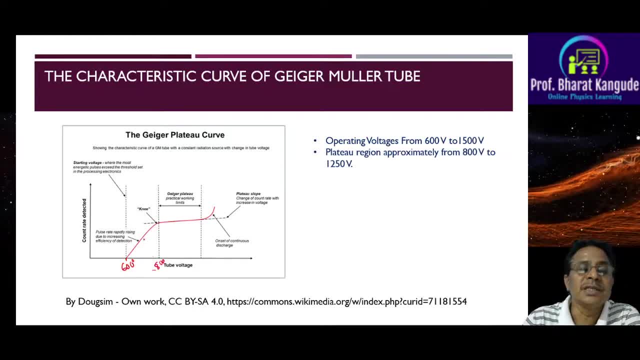 800 volts or like that, and in this this region is again not useful. So this is called as pulse rate rapidly rising due to increasing efficiency and of detection. That means our tube starts detecting such type of incident particles in a very fast way and that's why it starts detecting this type 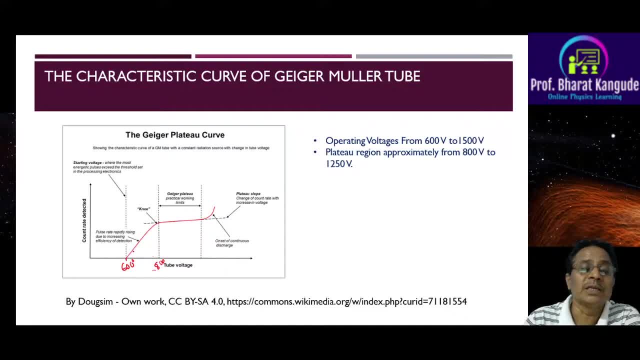 this start detecting or showing this type of electric pulse which is showing here. So this pulse rate rapidly increases. This is pulse count rate, or pulse rate detected. This increases as shown here, and there is certain potential, called as knee potential, where when we increase this, 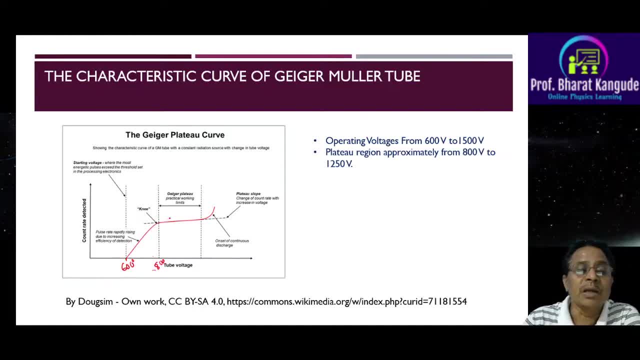 potential. beyond that, then, the number of particles counted are directly proportional to the number of particles coming in. Here this number of count is proportional to voltage. Here this is not proportional, but this number of particles counted by this type of counter, This is directly proportional to the particle coming in. and this is the region which is called as plateau region. 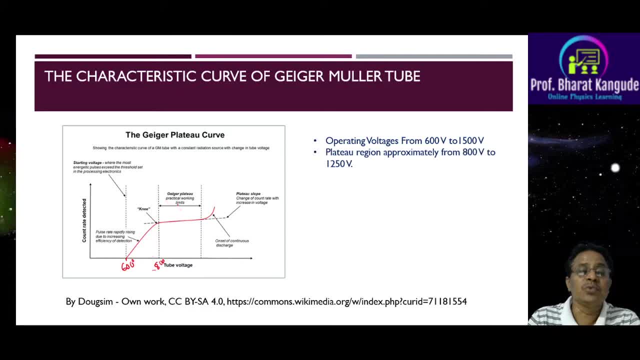 for this type of gm cube and this is the region we have to use for the working. actual gm2 works in this region that is called as geiger plateau. Practical working limits are shown here For different device. these practical limits may be some here and there but we can understand Usually. 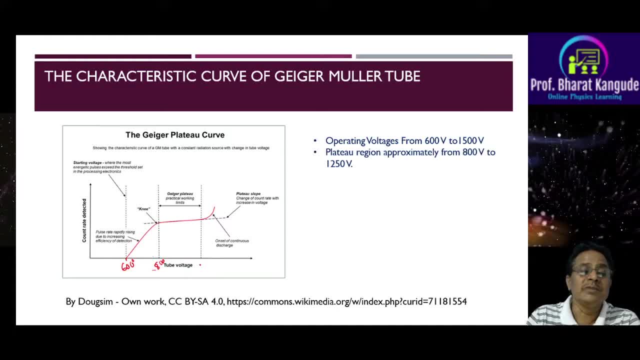 for almost all types of gm counter. this limit is from 800 volts to 1250 volts somewhere, so this particular voltage range is said to be the suitable and useful range for the measurement of this type of incident particle by this device. on the right hand side as we start. 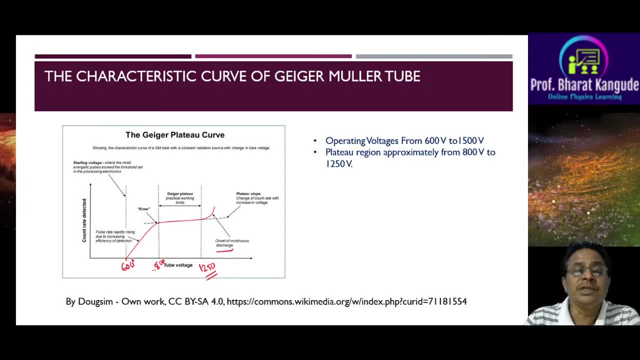 increasing this voltage. now there is an onset of continuous discharge. that means without this particle incident, such type of particles incident upon here because of very high potential, almost for 800, 1600 volts etc. this automatic discharge of material medium inside that tube takes place and then secondary, tertiary electron generation is there and thereby count rate again increases. 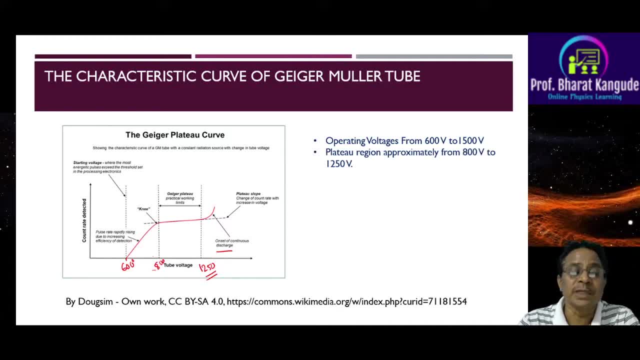 very fast, which is independent of the process that is happening inside. so this type of region is also to be avoided and therefore we have to go for this region, which is shown to be a plateau region, that is, that means operating of this particular gm tube is to be usually done in this plateau region. 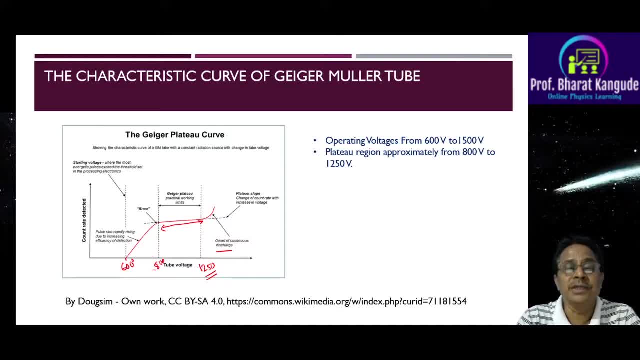 where we can measure accurately number of particles that are incident in this process. and then there are types too. so, once again, remember this. operating voltage is from 600 to 1500 volts. plateau region is approximately from 800 volts to 1250 volts, depending upon the type, depending upon the manufacturer, depending upon the 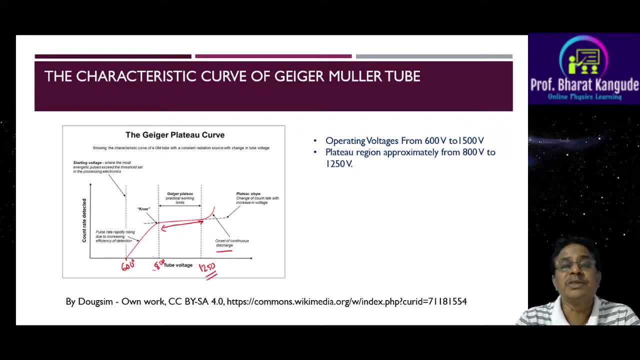 particles which we are supposed to measure there. this, this numbers may be somewhat here and there. these are the initial values, or the values of this such type of gm counter, which was produced by, initially by, these people. then there is one more important aspect we have to learn here. 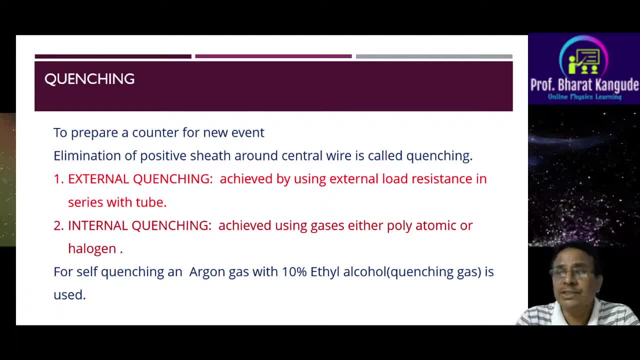 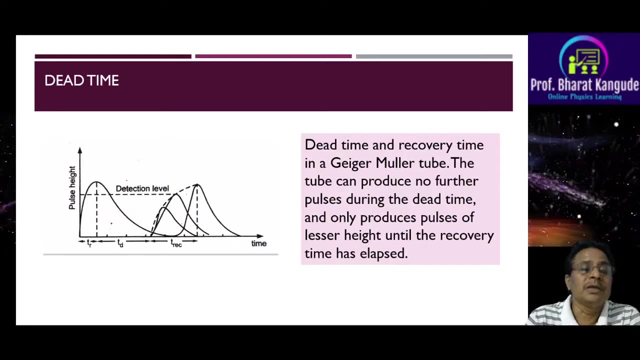 this is called as quenching. what is this quenching? quenching is another very important process that tells you how much efficient your gm counter is. that means in this process. so for that we will just go for this next figure here that shows you this particular part here, that that shows you this. 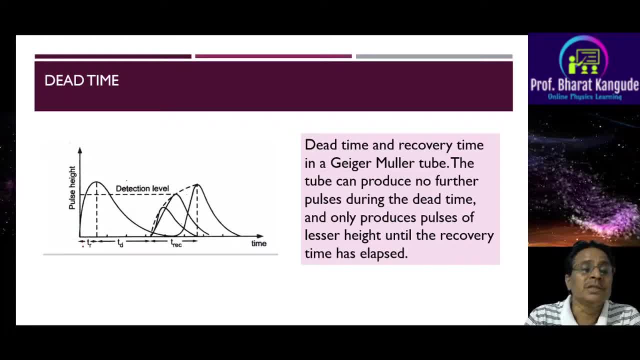 is full height. whenever certain radiation comes in, the false height rises abruptly, very right. this particular time is called as tr. it reaches this, this tr or this pulse is reaches at this height. now it starts falling here immediately. after certain time it reaches to some minimum here and beyond that, that is, before this. 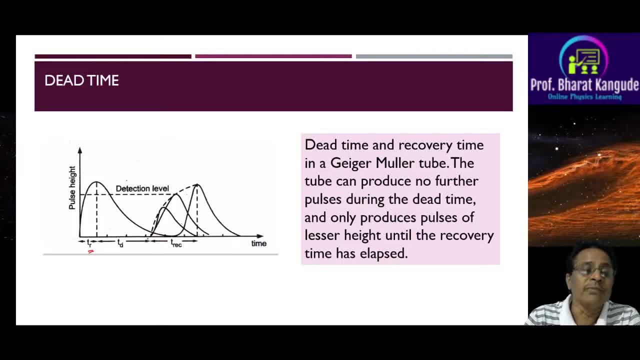 particular pulse goes off, goes off. there, there are some other types of particles are coming in, some other particles are coming in and they are also giving rise to a certain types of poles, as shown here, and you will find that, as this particular process of continuous discharge of gas, 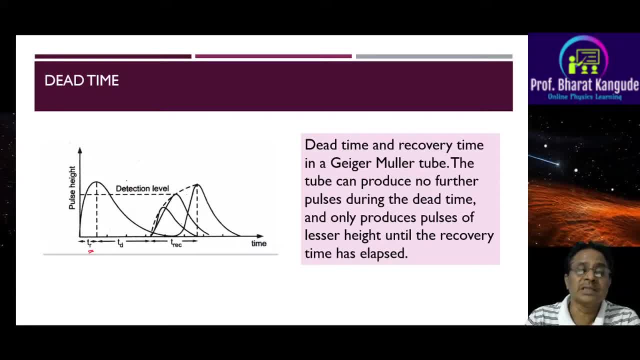 the atoms of the molecules of that particular gas- discharge gas like argon- to become ready for next type of particles. some time is required there. that is called as recovery time. so almost this particular, uh, this particular device or detector is a dead for this time which is called. 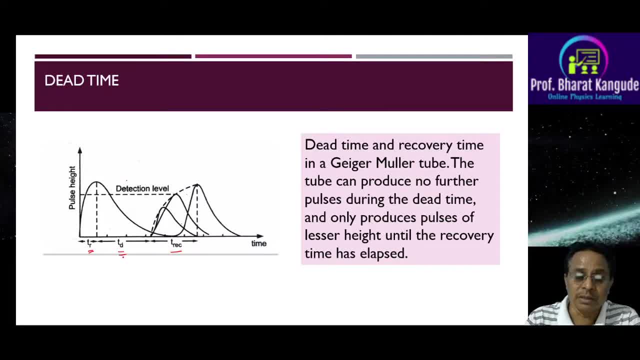 as this dead time of this type of uh detector and addition of this td plus t recovery. this is the time which is called as the uh, the time we are required here to make it a available for the, the uh next particle to come in. so dead time and recovery time in geiger-muller. 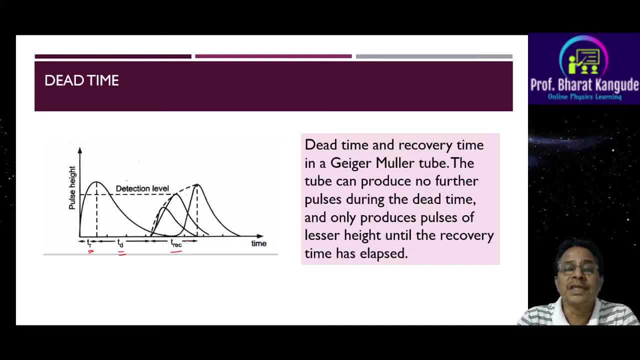 tube that you can produce no further pulses during the dead time. that means during the dead time when some other particles comes in that won't be counted, and that is what a lacuna of this particular problem. we have to reduce this dead time as far as possible and to reduce this dead dead time we 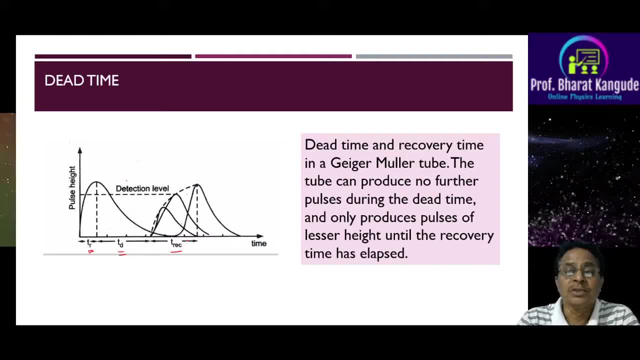 have to use the process which is called as pinching so and only produces pulses of laser height until recovery time has elapsed. so this secondary pulses, these are. these pulses are not actually because of the particles coming in, but these are from the internal processes are going on. 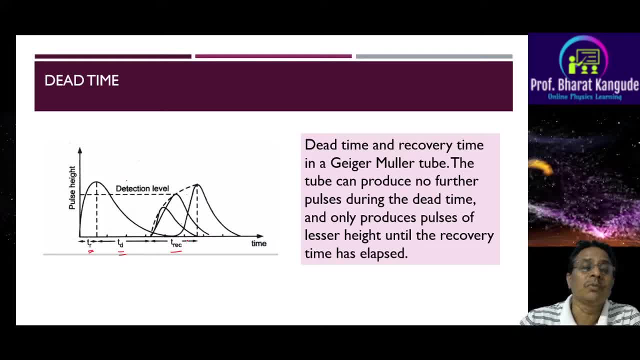 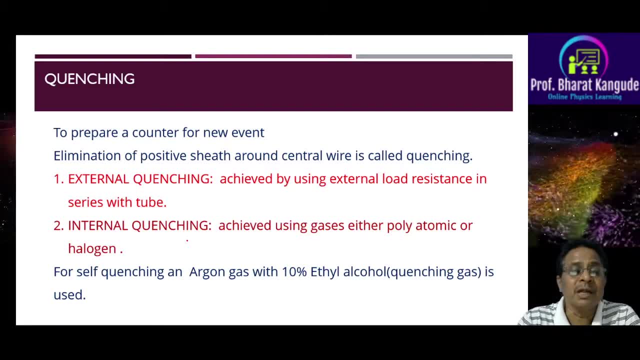 and to make this part as small as possible, we have. we require the process that is called as pinching, so once a particular particle comes in, a pulse is generated for accepting next particle. we have to prepare. this device has to prepare again so to prepare a counter for new event. 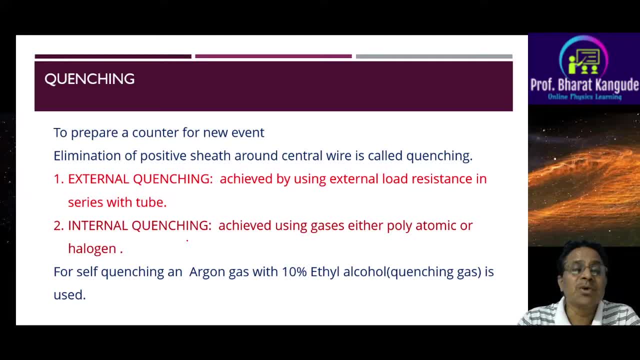 this pinching process is required. so this is the process which is carried out here. it is elimination of positive sheath. that means, whatever around anode, a large number of positive ions are there, this positive sheath of these ions, and this is to be shifted, or this is to be neutralized, and this process is called as: 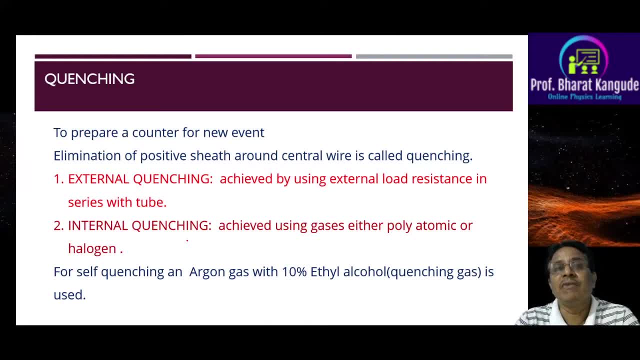 pinching. so elimination of positive sheath around central wire is called pinching. so we have to eliminate this type of positive sheath, otherwise there is a problem in electrons reaching towards this anode as well as ions that are reaching towards this cathode. there is a problem two ways. one is called as external. 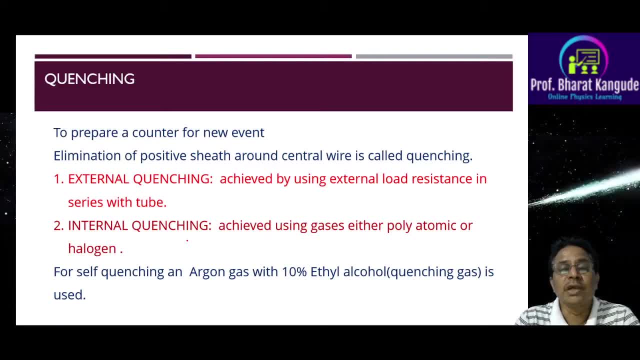 pinching achieved by using external load resistance in series with the tube. usually, this type of process is not used in case of this gm2. second method is more preferred here: internal quenching. that is achieved using gases, either polyatomic or halogen, and most of the time, as we have said, 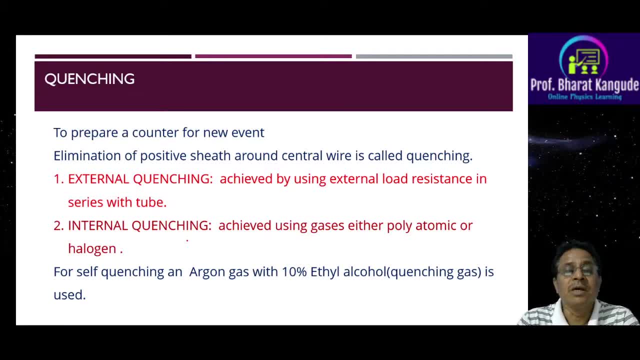 most of the devices that use self-quenching process, wherein we have argonic gas, gas that undergoes discharge with 10 percent ethyl alcohol that works as a inch quenching gas that is used there. so these particular ethyl alcohols, they neutralize this argon gas very. 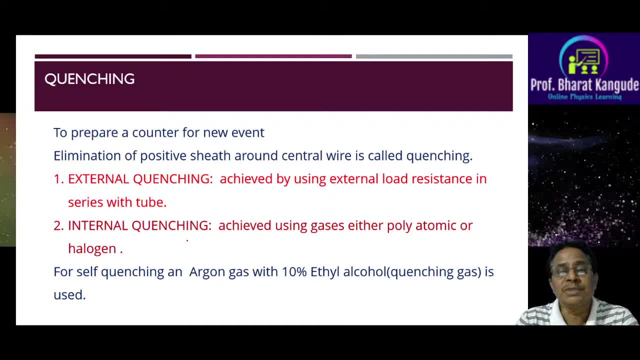 immediately and therefore this complete apparatus becomes available or becomes ready for the next particle in. and that's how this recovery time and this dead time, this can be made as small as possible and thereby this efficiency of this type of gm cube can be increased. so this is what the 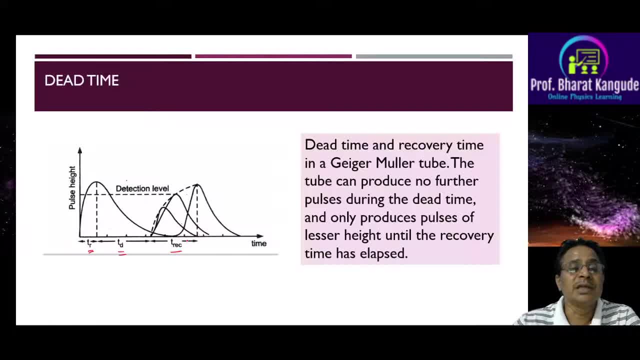 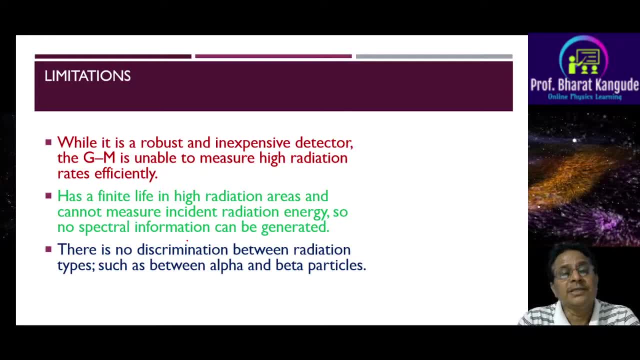 gm2 is. it is working and the functioning of this type of gm2. it has certain limitations and there are certain applications that we are going to see here. so what is one limitation? why it is a robust and inexpensive detector. so this is very easy. it's cost effective. no higher cost is required for that. 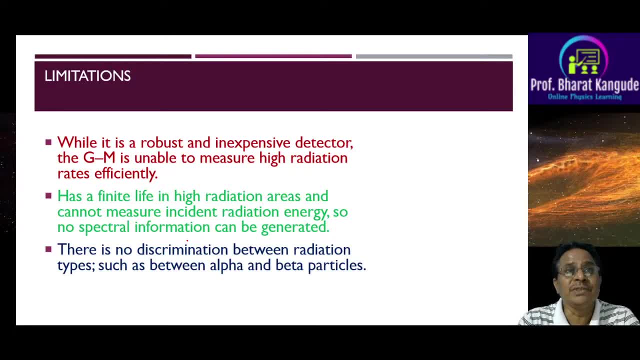 the gm tube is unable to measure high radiation rates efficiently. as i said, whenever certain new radiation, if the number of count is very, very large per second, if thousands of radiations are- are coming in, then it is very difficult for it to measure this number accurately. that 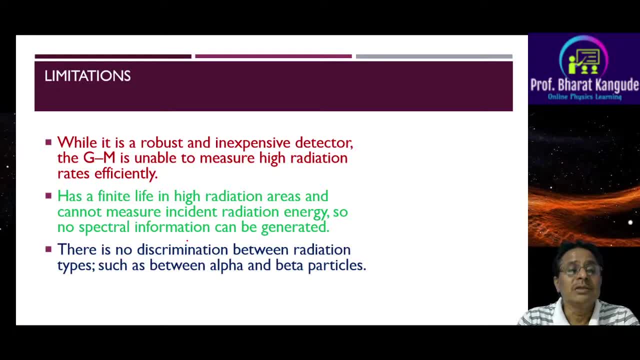 is what one lacuna or one limitation here: This type of tube has a finite lifetime because of the quenching process of the gases, gases inside this tube that continuously it goes in by quenching process and that is why a finite lifetime is for that. 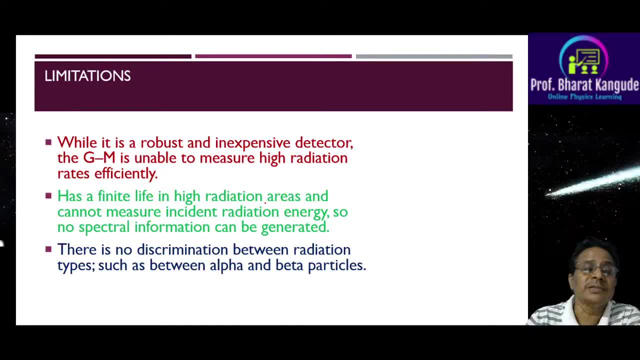 So how has a finite life in high radiation areas and cannot measure incident radiation energy. So it cannot measure this energy of the radiations coming in. it just measure, counts the number, it counts the number and it doesn't count the energy of the particle incident. so for 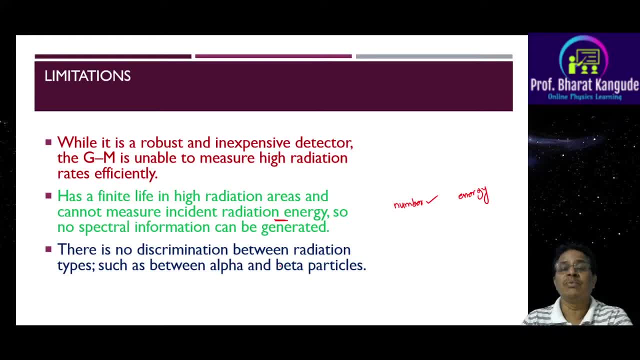 that we need some other device which will measure energy of such type of radiation that are emitted in such type of nuclear reaction. So no spectral information can be generated. So if there are large number of particles are coming in, so if some particles have very low energy, some particles have very high energy, so this type of spectrum of particles cannot. 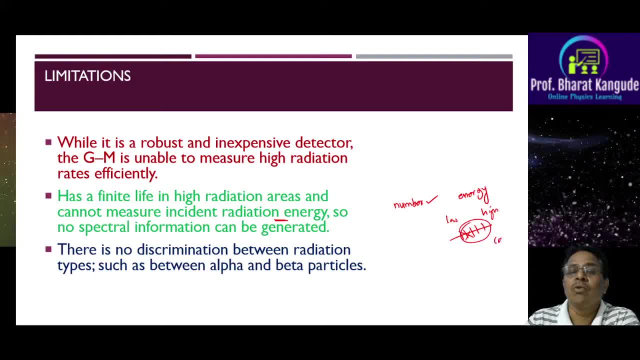 be generated. in this case, only this measures the count. what are the total number of particles coming in or incident at this stage, at this particular time? and there is no discrimination between radiation types, such as between alpha and beta particles. so this particular counter that that doesn't discriminate. 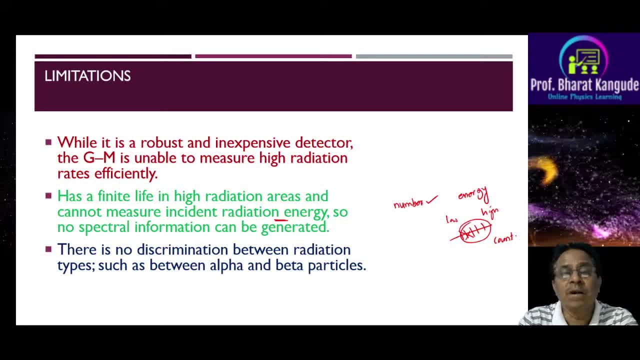 So if there are large number of particles are coming in, so if some particles have very low energy, so there is no discrimination between alpha and beta particles, so that only counts- some radiations are coming in, or there is some nuclear radiation which is observed, of this particular type and provided we have a such a very high voltage range, that works. 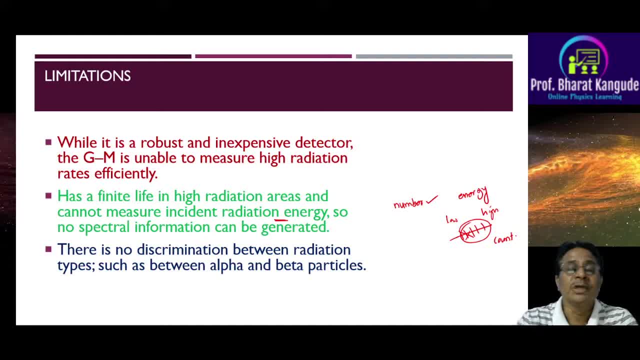 around 600 to 800 or 1000 volts and so on. so this exact working of this type of device, its limitation, its functioning etc. is interesting one, and this, this particular device, has large, many applications. Probably this was the first device which was prepared for this particular type of radiation. 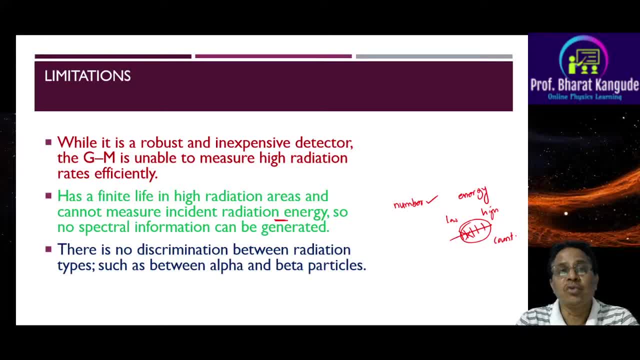 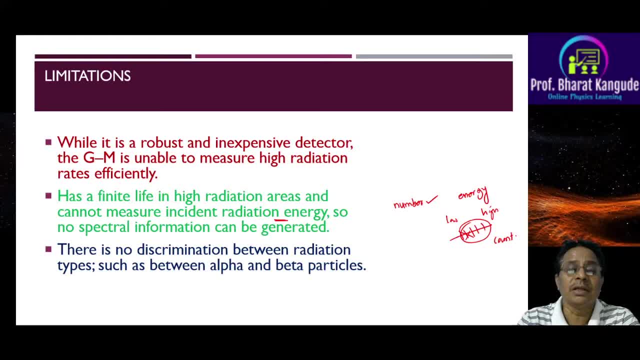 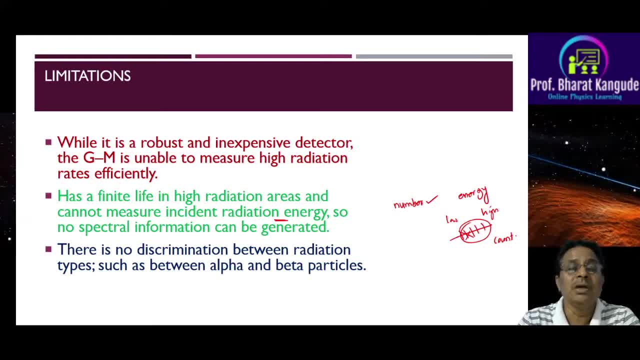 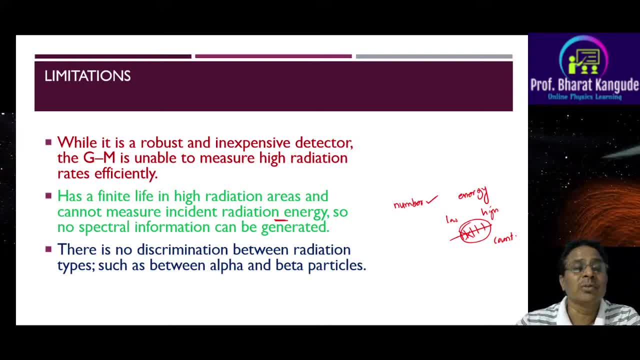 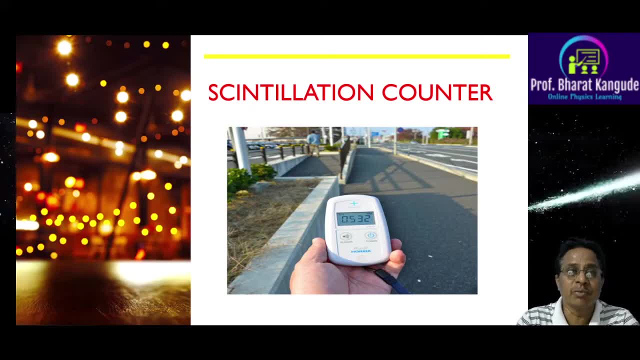 Probably this was the first device which was prepared for this particular type of radiation things. So here we have finished this first part of our presentation. Now we will go to the second Now. first was the gas ionization type of device. Now this is the scintillation counter, which is 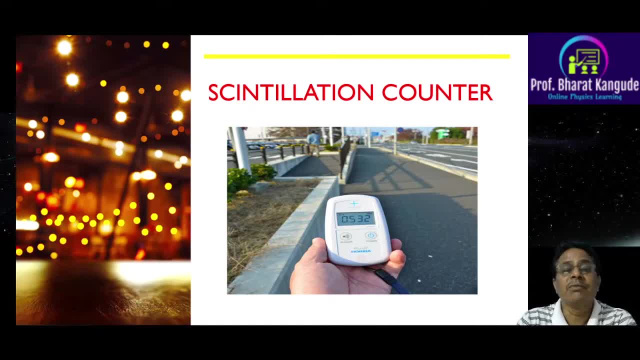 usually using this solid state material for the process of interaction of this incident radiation with the material medium. This is one very small handhold device. shown you where it measures this count: 0.532 somewhere and this is plus sign that shows actual counter is here. This is what all electronic assembly, with that There is a start and stop button Whenever. 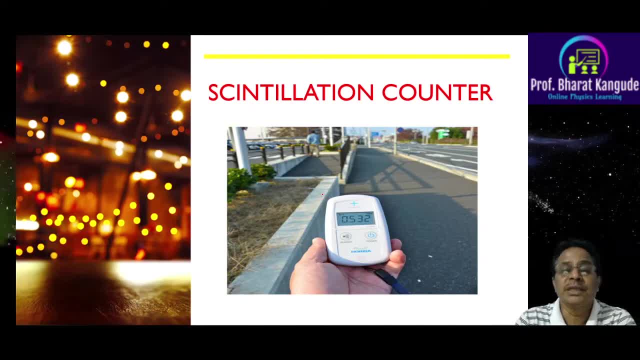 we start this button, what are the number of radiations present in that case? that will be counted by this counter. and this is one very simple handhold device which can be very nicely used for detection of this type of particles or the radiations as we can see in this particular diagram. So before we go for actual study or the description of all, 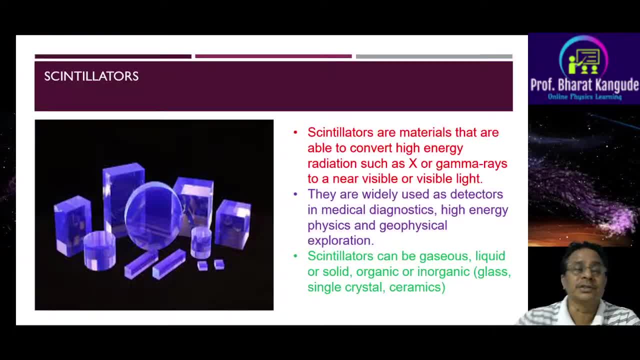 this type of devices. let's see what do you mean by scintillators or what do you mean by scintillation process. Now this diagram shows there are some glass type of materials. What these materials are made up of. Some of them are organic, some are inorganic, some are glasses. 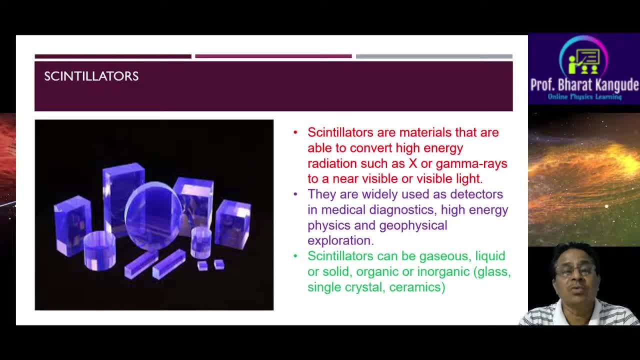 some are plastic and lot many types of materials are there. So what do you mean by scintillators? Scintillators are material that are able to convert high energy radiation, such as X-rays or gamma rays, to a near visible light. So these radiations, that these particular particles are, incident upon this material. 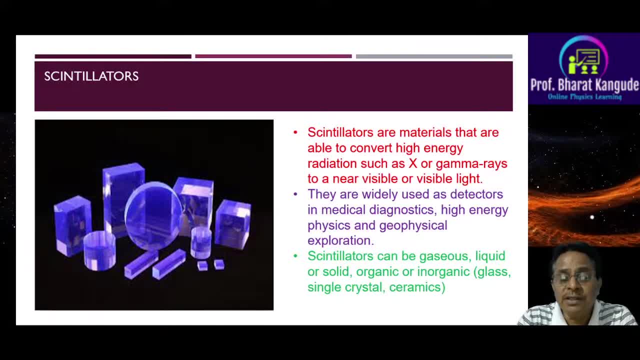 there happens an interaction and radiations and in the visible spectrum or electromagnetic spectrum near visible, these type of radiations are emitted by these type of materials. They are widely used as detectors in medical diagnosis. So in medical diagnostics these materials are frequently used in high energy physics. 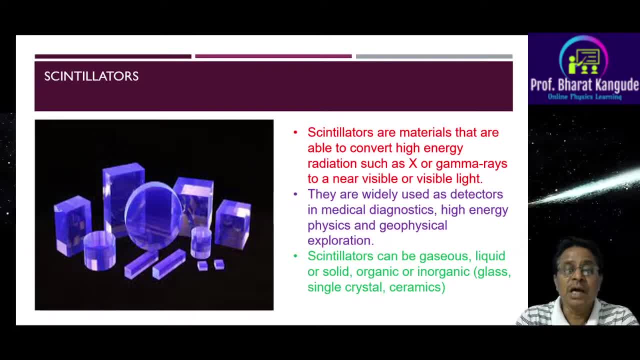 and geophysical exploration. So these scintillators are used in different devices where, either for geophysical exploration, in medical physics, in high energy physics, where incidence of such type of particles can be obtained or can be understood very easily using these type of counters. 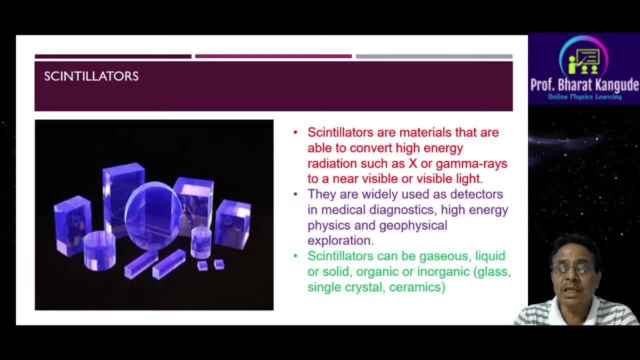 Now, scintillator materials can be gases, can be liquid or solid, As well as inorganic glass, single crystal or ceramics. there are several number of other examples which can be shown to be showing these type of properties and, depending upon what type of scintillator we need, either we can use solid, we can use liquid, we can use 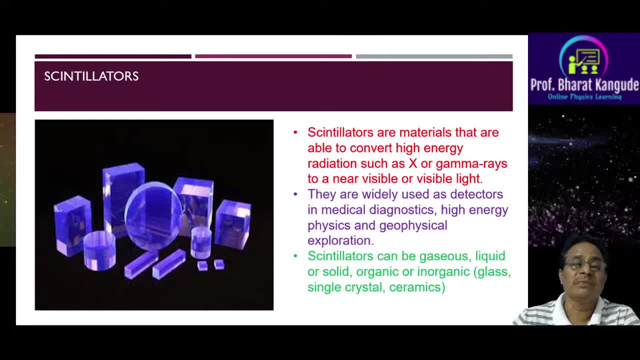 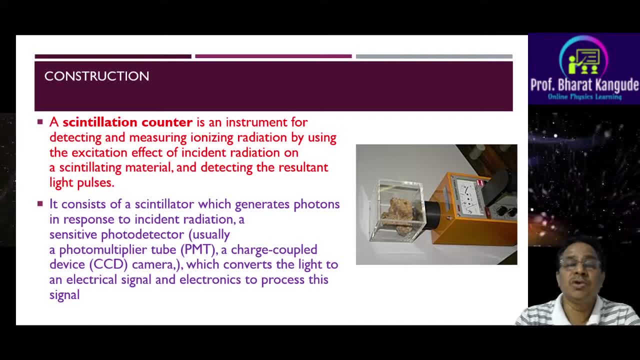 gases. that is a choice of a particular manufacturer, of what type of scintillator that particular person is supposed to produce. Now, this is what one simple device- you have been shown this diagram- tells you. this is the part here. this is actually uranium salt. so this is a uranium salt which is kept very 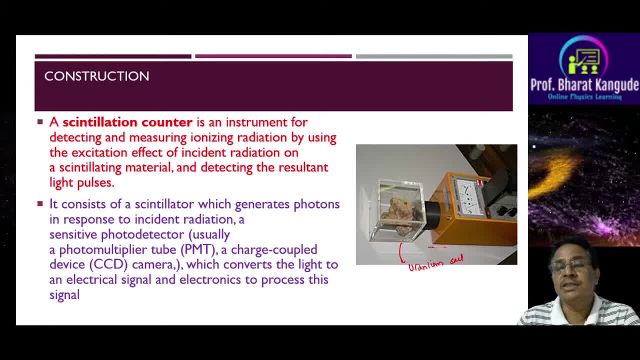 close to this particular device and this is our device, which is called as scintillation counter. Here this actual process goes on with this radiations and this particular scintillation material and all these are electronic parts of this- which measures and counts all these things and so on. 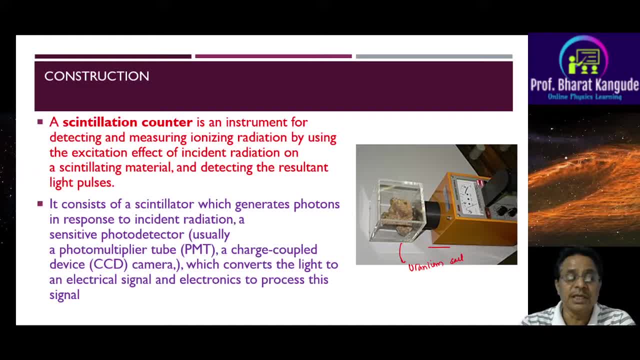 Now let's see this construction. we are going to see its detailed diagram in the next slide. A scintillation counter is an instrument. It is an instrument for detecting and measuring ionizing radiations by using the excitation effect of incident radiation on a scintillating material and detecting the resultant light. 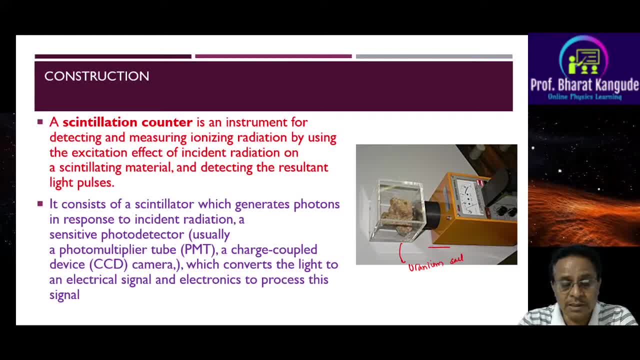 pulses. So some light radiation incident that interacts with this type of material- scintillator material- and that produces the photons and this such type of light pulses are generated. These pulses are used further. It consists of scintillators, Which generates photons in response to incident radiation. 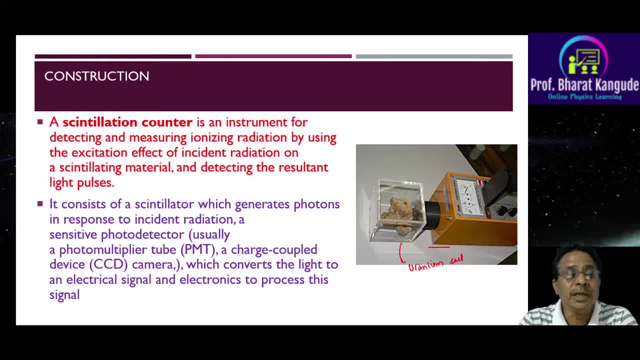 Alpha, beta, gamma is coming and photons are radiated. A sensitive photo detector, usually a photomultiplier tube, that is PMT, A charged coupled device and sometimes that is CCD camera etc. are connected further, which converts the light to an electrical signal, and electronics to process this signal. 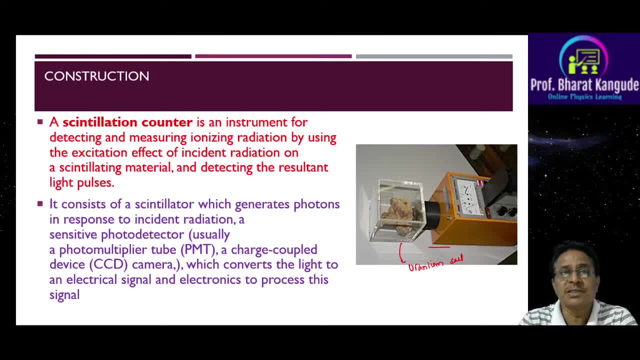 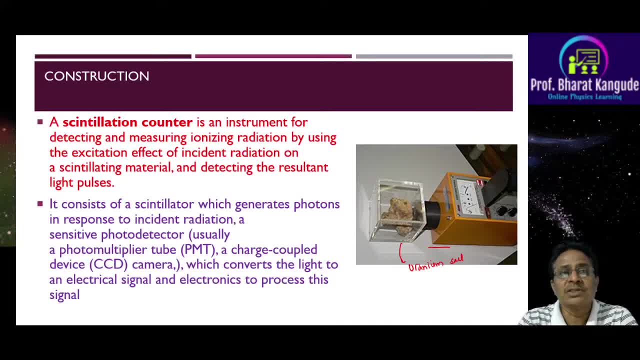 This is the photocathode, So this is the photocathode. This is the photocathode, So this is the photocathode. So this is the photocathode Which emits electron. and once this single electron is generated further, this is amplified. 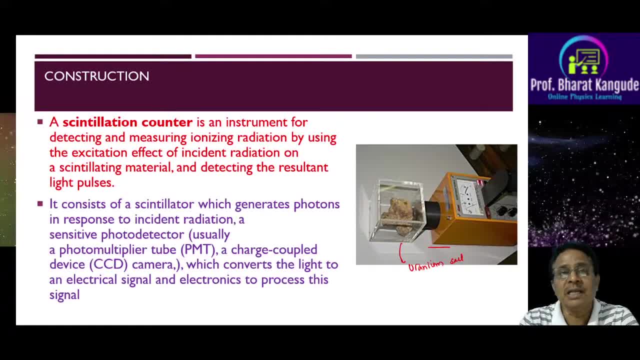 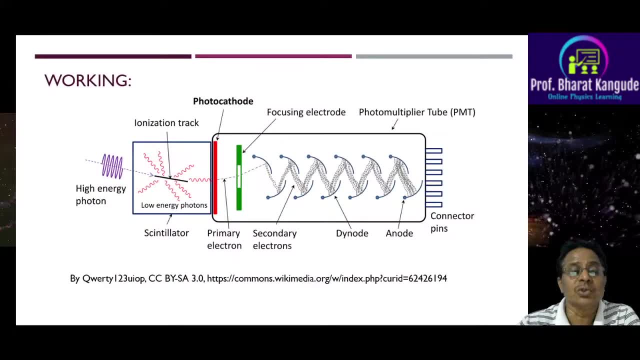 by a process and a large signal is created and that can be counted very easily. and that is what this entire operation is there. So the device is shown, Its construction is also shown there. This is what the good diagram that shows you how actual working of this particular thing. 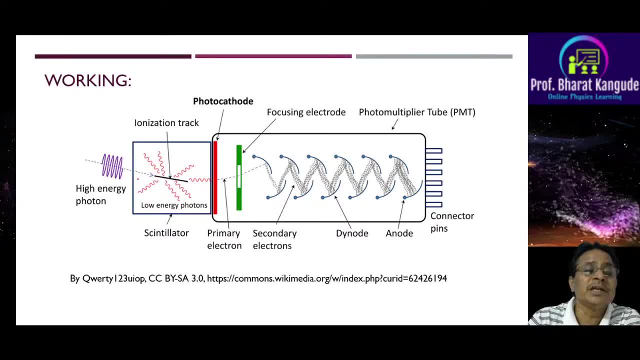 comes here Now. that shows this first part. This is called as scintillator. material is here. This is the part which is called as photomultiplier tube. in this photomultiplier tube, this red part is shown to be photocathode. this, this green part. 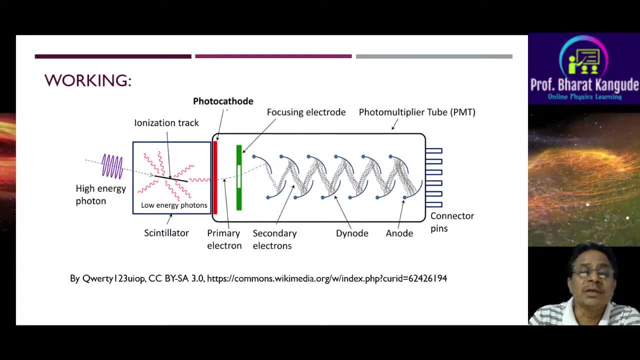 is shown to be focusing electron and these, these curved surfaces, this is first, second, third, fourth, etc. these are said to be dianodes. okay, all these are said to be dianodes and last dianode is called as anode. so positive of the battery is connected here and negative of the battery is connected to. 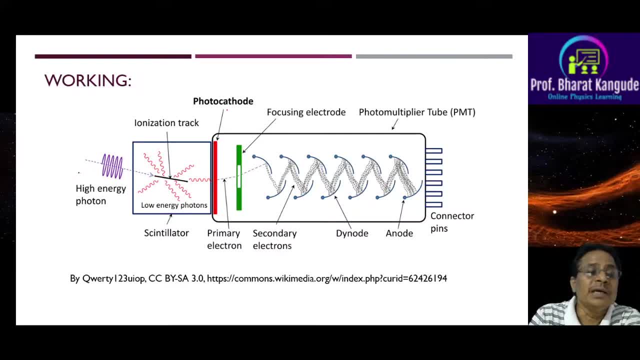 this photocathode and now, when this incident, high energy incident particle comes in, this particle interacts here with this particular material medium. whenever it is passing through this, it produces this type of protons, some of the photons, directed toward this photocathode. this photocathode is a material which emits an electron, the primary. this is called as primary. 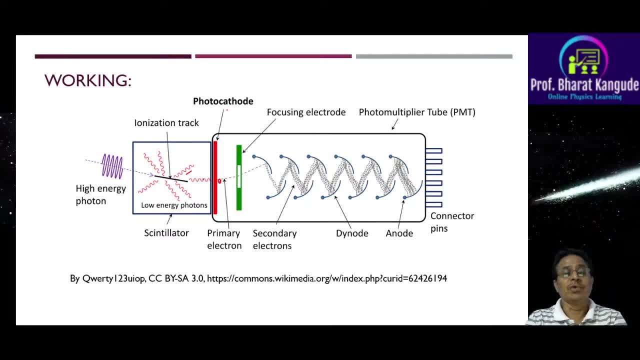 electron is emitted here. because of this interaction of the photon, high energy photon, this photoelectric effect takes place at this photocathode. okay, this type of electrons which are emitted here, these are accelerated towards this and passing this, focusing after focusing, it falls on this anode. 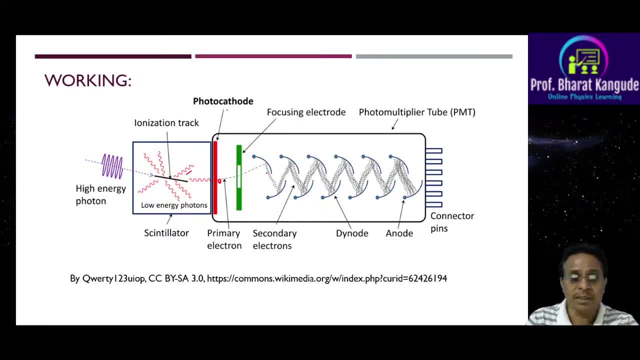 which is a positively charged part here. because of that this electron gets accelerated. here it produces more number of electrons. further, these electrons are accelerated among towards another anode. here also the process of multiplication takes place. so one comes, two comes there, then the three, then five, then seven, then eleven, like that. 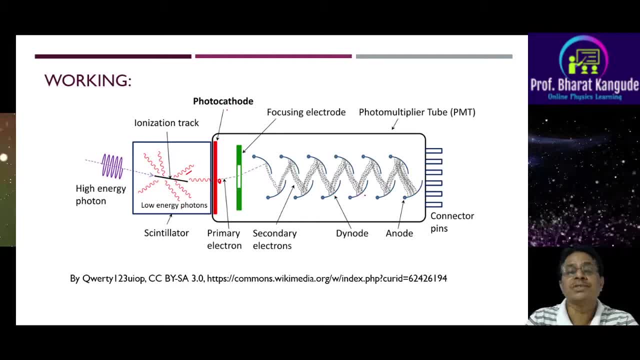 this number of electrons emitted by every of this anode goes on increasing. and, lastly, these electrons are collected by this last anode and which gives rise to a sharp pulse. electrical current pulse is observed as a response to this incident particle. there, that is when single particle comes in. 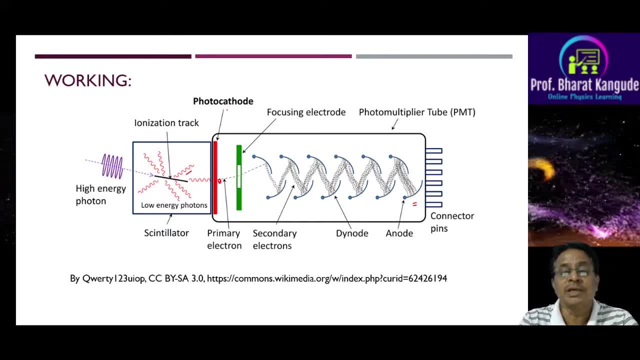 such single type of pulse of a high voltage will be generated and thereby measuring such type of pulses, we can determine how many number of such particles are incident there, and this is what the functioning of this type of the device, which is called as scintillation counter. 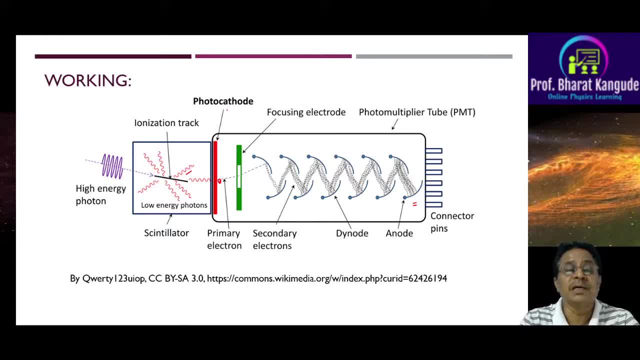 so this scintillator materials. this interaction takes place in this material. in the scintillator, photons are generated, photons are incident upon photocathode, which generates electrons. further, these electrons are accelerated and more and more number of electrons are generated to give a sharp pulse. and that's why this second part of this device that is called as 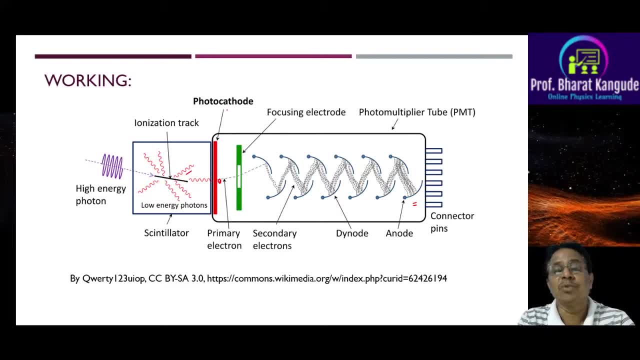 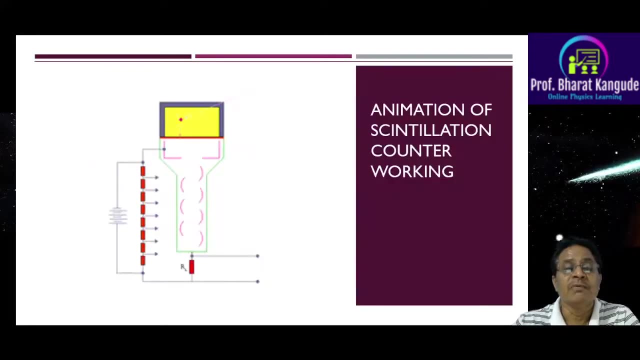 photomultiplierty. so whatever electron generated because of this photoelectric process, these electrons are amplified and a measurable signal is generated. based upon measurement of these signals, we can measure how many number of such incident particles are there. so this is the functioning. further it can be shown. this is one very nice animation that. 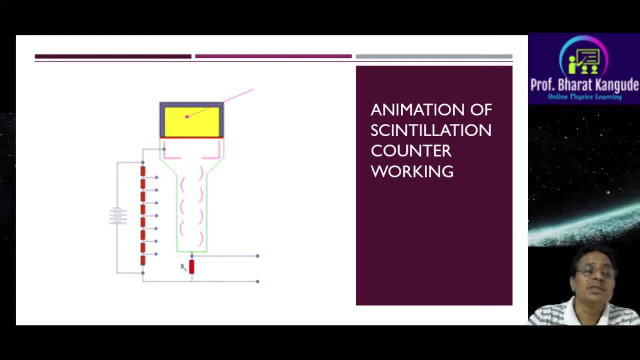 shows you how this entire process goes on. look here, this is incident particle coming in. this interacts with this material medium particle. here generated this photon incident upon this photocathode. this electron is shown here. further this electron. now look at this everywhere. this this is connected, this is connected to this. 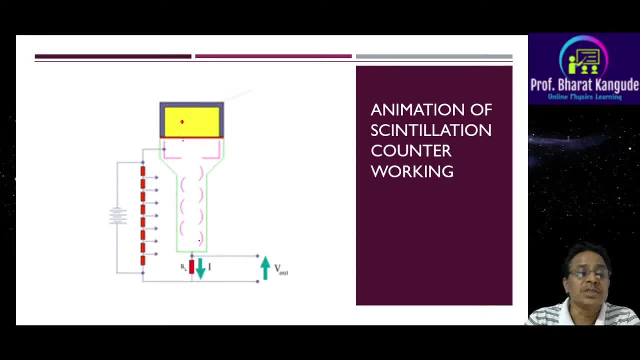 negative part and this is connected to this positive. so this is what a last anode shown here, which is connected to this positive of this battery. high voltage is there and initially, when this electron comes, single electron multiplied, gets multiplied, gets again multiplied, like this, and that shows a large number of electron, binary, and it's a small pulse. this type of pulse is: 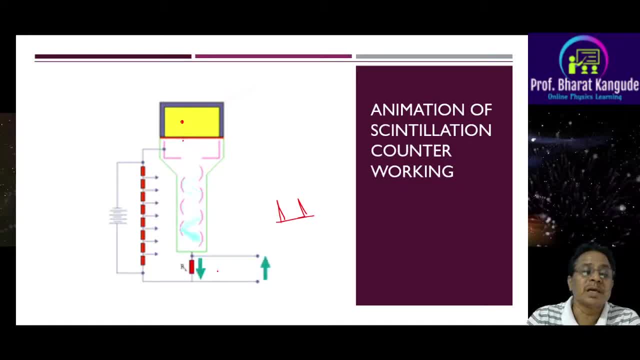 generated after certain regular interval. as this particle coming in, these type of pulses are created. and measuring these pulses we measure the number of such particles. incident there. so count is to be measured. so this is also a counter that doesn't detect, tells you whether it is alpha. 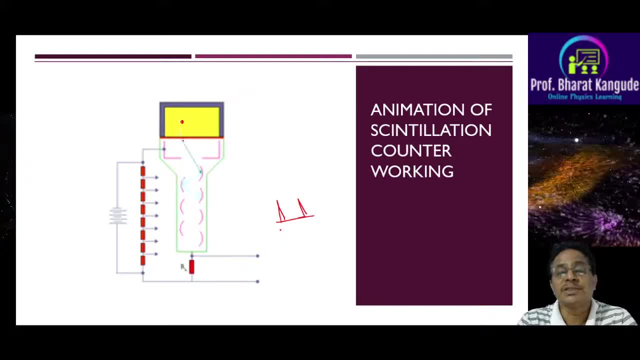 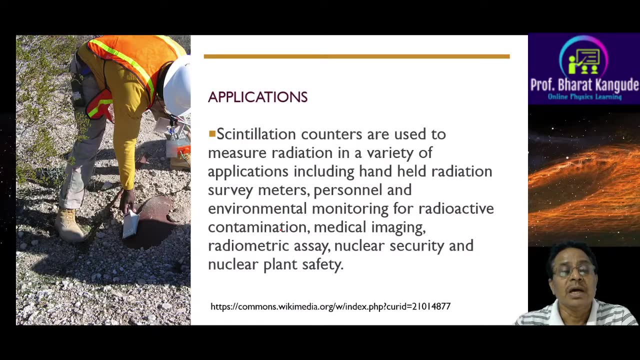 particle or beta particle, but it detects how many such type of incident particles are there, so nuclear radiations which can be measured by these type of devices, that it also plays a very vital role in the in the measurement of such type of particles or such type of things here and now. let's see here how this is a particular person. 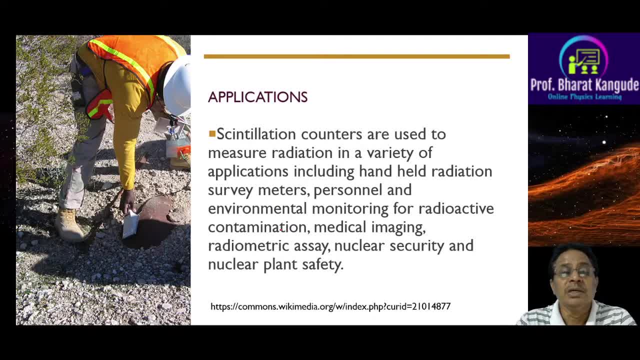 who is using this type of scintillation counter to measure something. so scintillator counters are to be used. are used to measure radiation in variety of applications, including handheld radiation survey meters. the person is showing in his hand personal and environmental monitoring for radioactive contamination. so in some cases we see in laboratory there are some cases of leakage of this radioactive material. 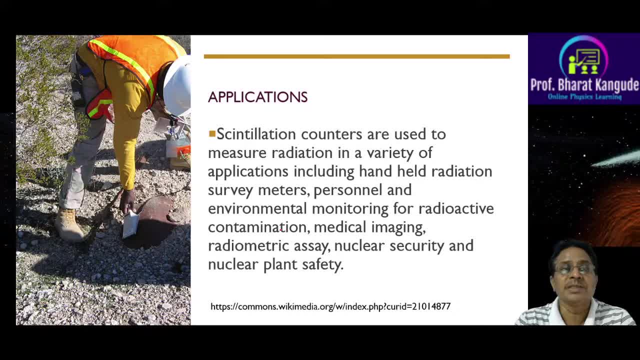 so where this leakage has been occurred or what is the amount of radiations there, whether it is hazardous or not. it is that this type of devices are used in medical imaging also. this type of devices are used radiometric assay, that is, survey, or the radiometric 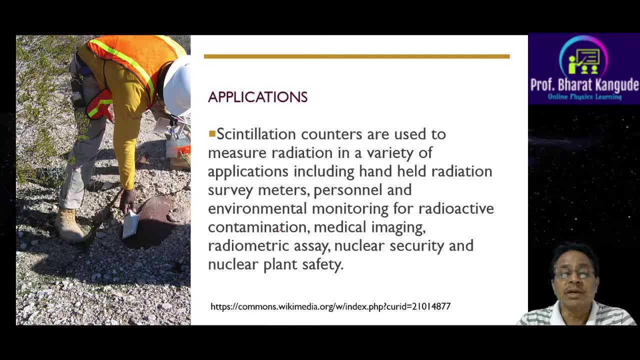 assay of a particular survey can be done here: nuclear security and nuclear plant safety. so this is one very simple, handheld, low cost device which is used to measure the number of radiations or the radiations occurring at any place, and thereby safety of the devices, safety of the places, safety of the human, etc. can be ensured here, and 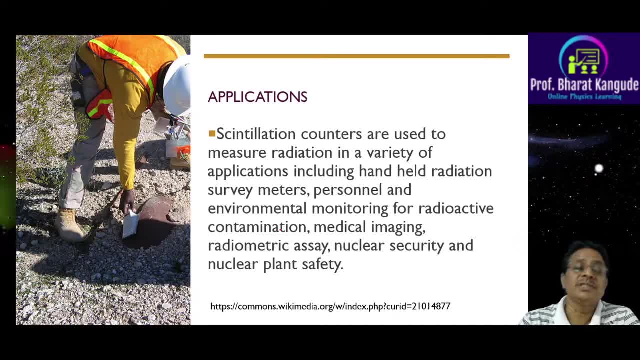 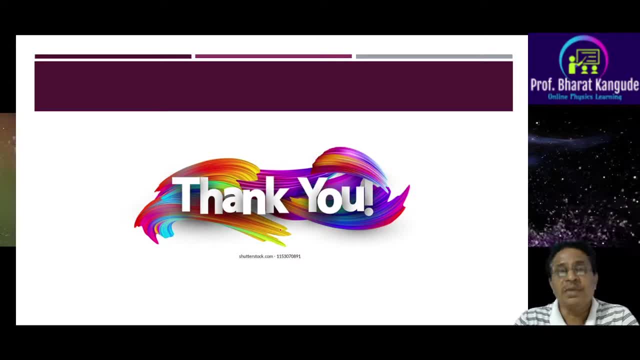 this is what a nice application of all these devices that is part of this scintillation counter. so apart from that, there are few more devices too. all other devices are there, and these devices also help in the process of detection of several different types of nuclear particles. 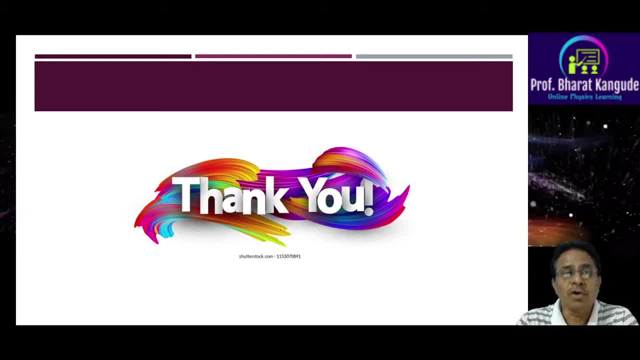 for neutron, we require require different types of detectors for neutrino. we require different types of detectors for alpha beta gamma. we can use some of these detectors. so, as well as how this nuclear physics is evolving or becoming richer and richer, this technology of the devices is also. 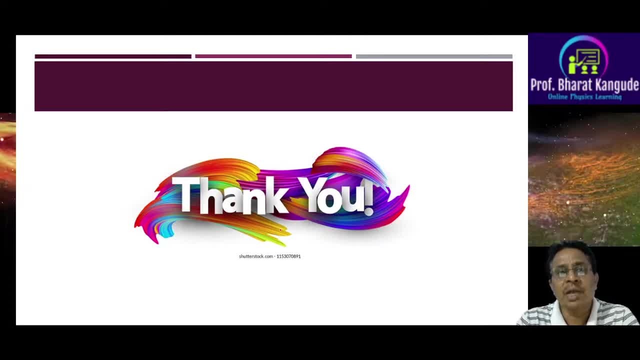 becoming richer and richer day by day. now very sophisticated hand-hold electronic devices are coming in which are very nicely used in nuclear physics all over the world for measuring such type of radiations and all these things. so in in our discussion we have shown two primary or basic types of detectors, but nowadays detectors 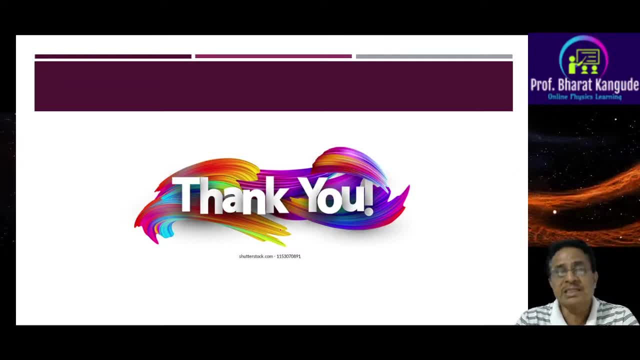 available in the market and which are being used very nicely in all such type of processes. they are found to be one of the ultra modern tools here. so that is how, in both of these stations, we have learned what are the accelerators. in this session, we have learned what are the different types of.